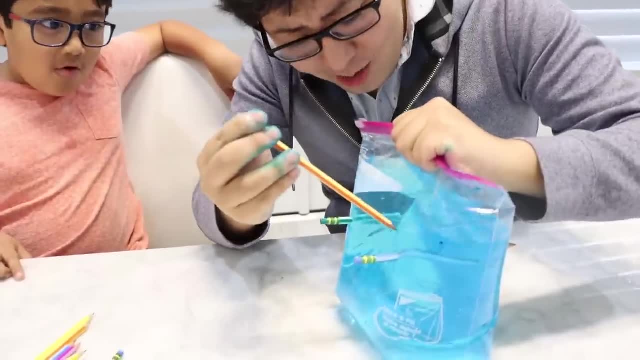 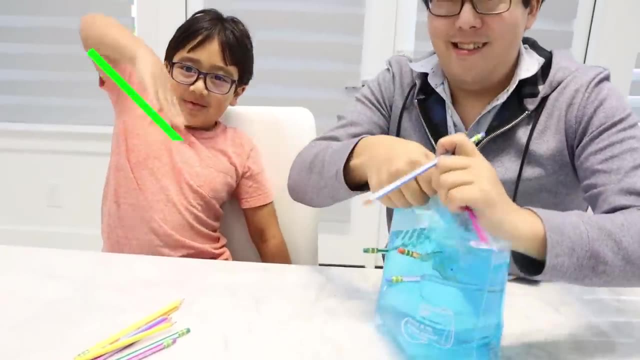 All right, let's see. I'm going to do it at an angle. Does it work? Whoa, Whoa. it works, Whoa, That's cool. Now you do it up and down. All right, I'm going to do it from the opposite direction. 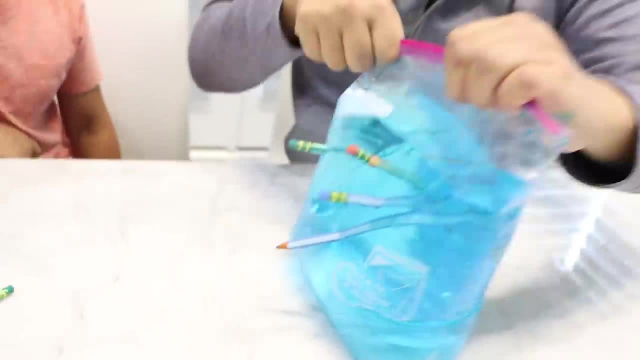 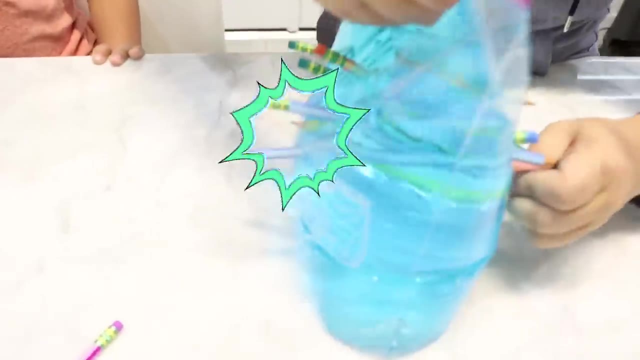 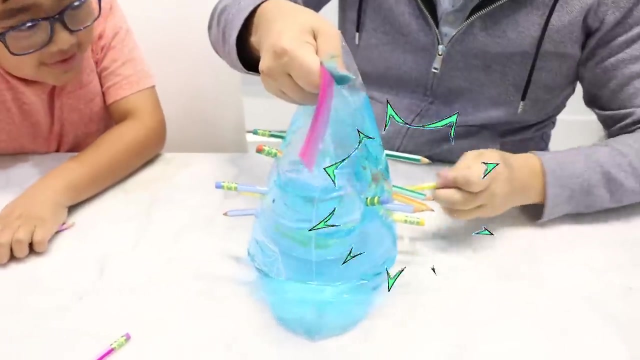 Up down. Whoa, Whoa, it's working. Yeah, it is. I'm going to do more. Whoa, Oh, Whoa, Whoa, Whoa. There's so many pencils. All right, I'm going to keep going. 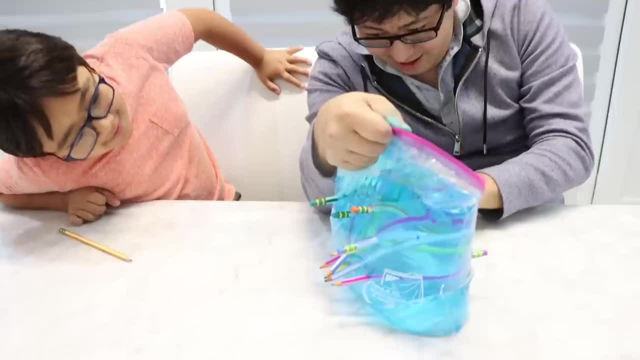 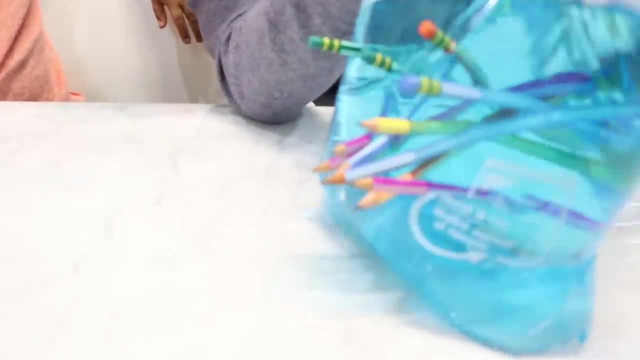 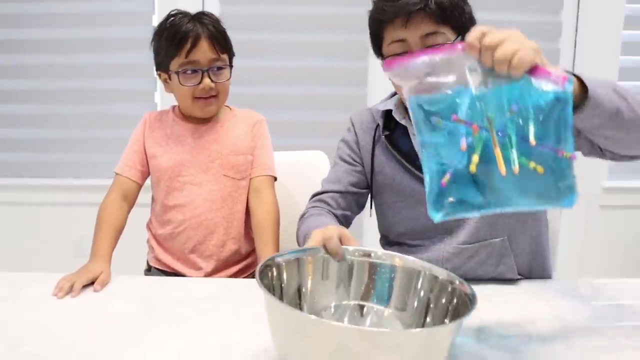 Let's see if I can do all of them. Ouch, I think I poked too much. What do you think, Daddy? what about we take out all the pencils and see what happens? Good idea, Let's put in the ball. 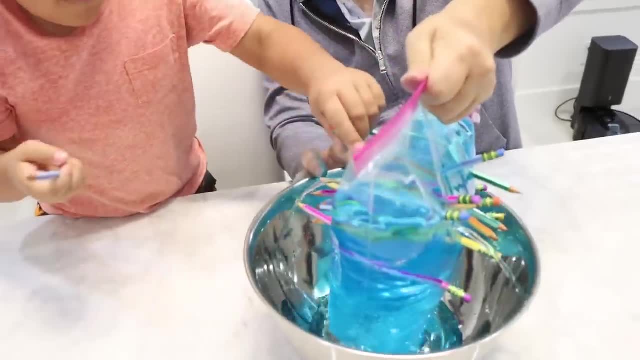 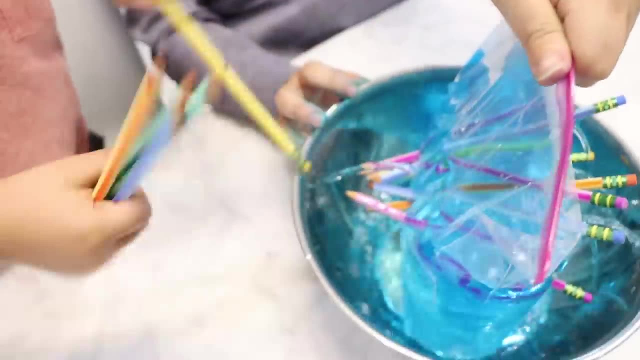 All right, Let's see what happens. Whoa, Water's coming out. Oh, There's so much water, Water, Water, Water. those Whoa Look at that. Well, there's so much water coming out, I could shower. 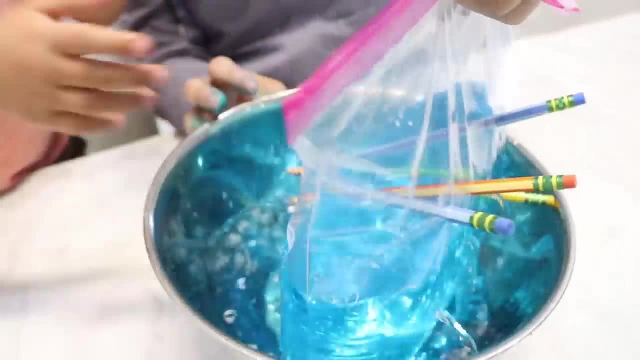 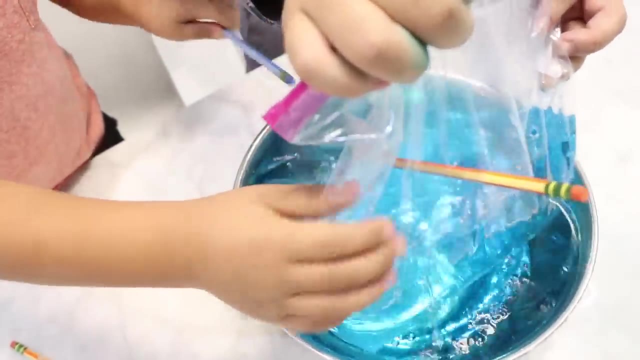 It's a waterfall of water. Whoa, There's so much. Oh, I am in the middle of this. Oh, There you go, There you go. Oh my goodness, Oh my goodness, Is this an elephant? No, 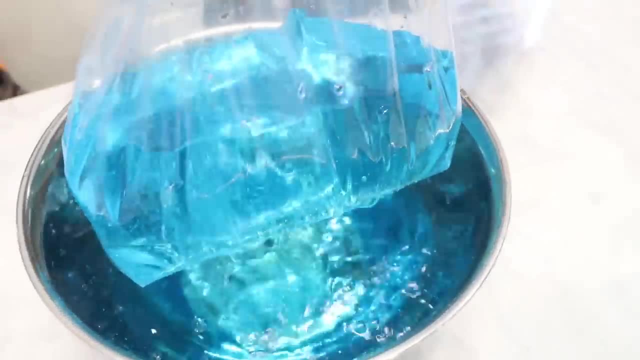 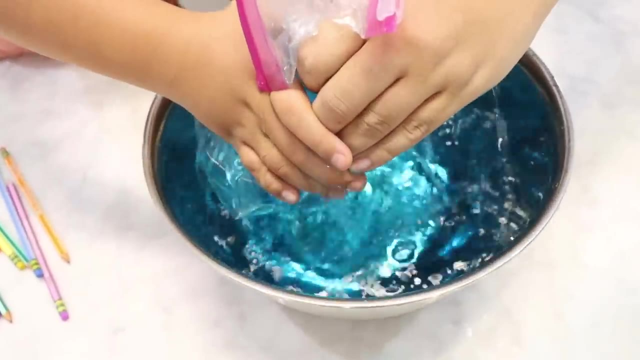 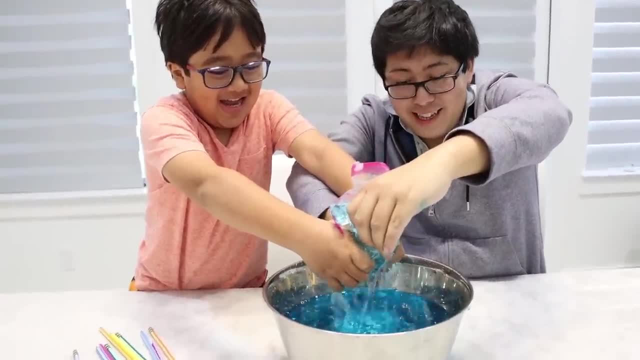 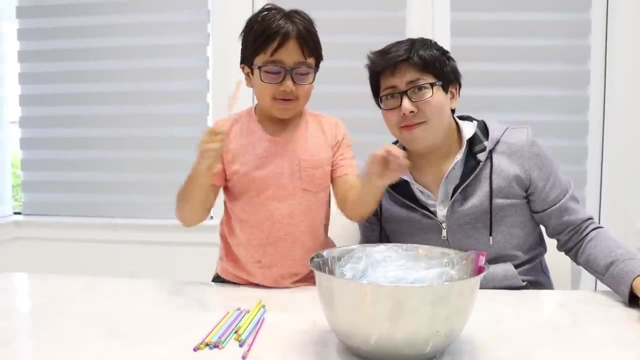 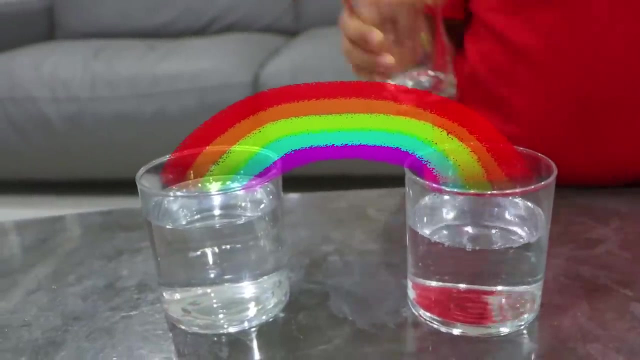 whoa, whoa, whoa big mess. Wow, it almost filled up the whole thing. Thank you for watching a science video about pencils and poking in your bag. Hey guys, today we're going to grow our own rainbow. All you need is a paper towel, scissors, markers and cups with water. 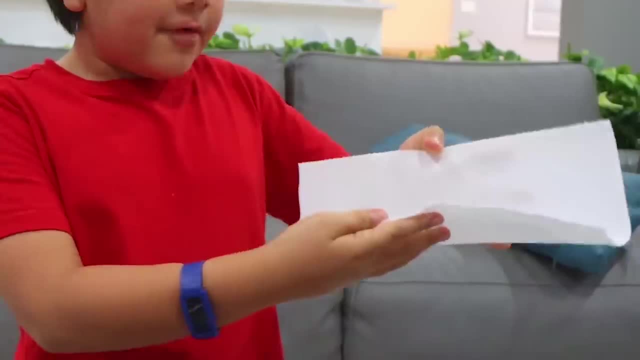 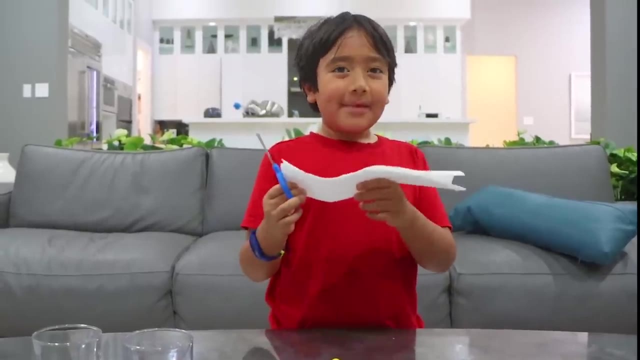 First, using your paper towel, you're going to fold it in half, and then we're going to cut a one-fourth. Don't forget to ask a grown-up for help, and I have mommy here. Hi, Hi, Thank you. 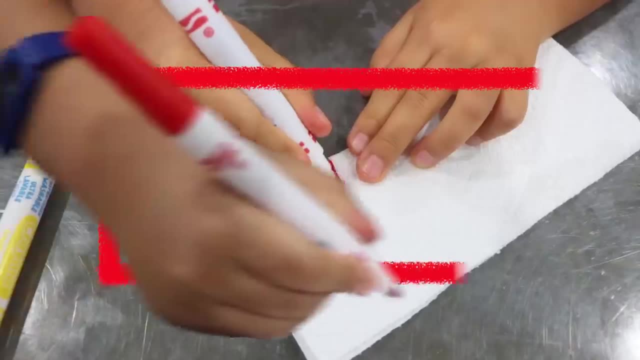 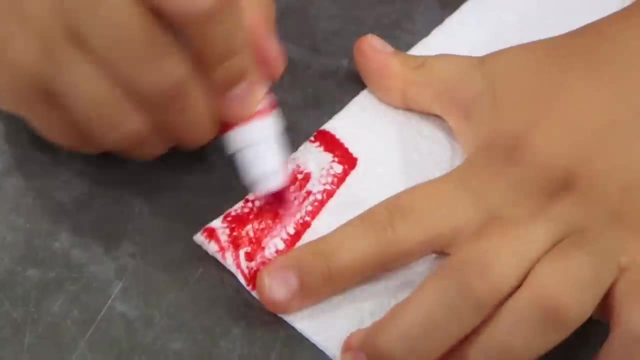 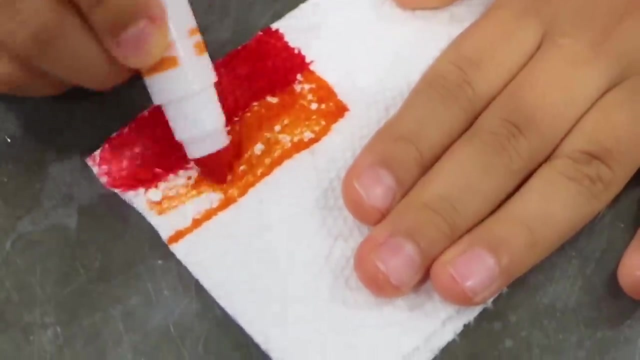 So first, with any marker you want, make a rectangle like this: Now let's cover it in. The next color, in the rainbow is orange, Put it like this: Now let's fill it in. Next is yellow. Okay, let's fill this in. 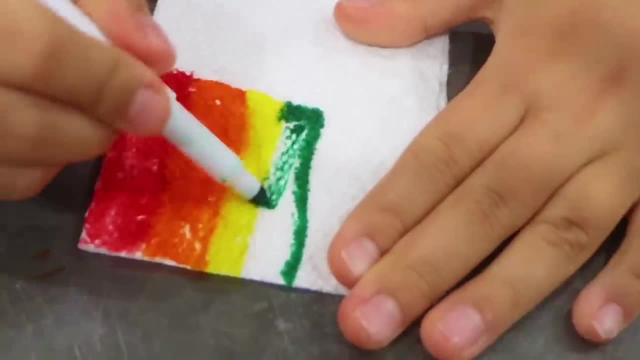 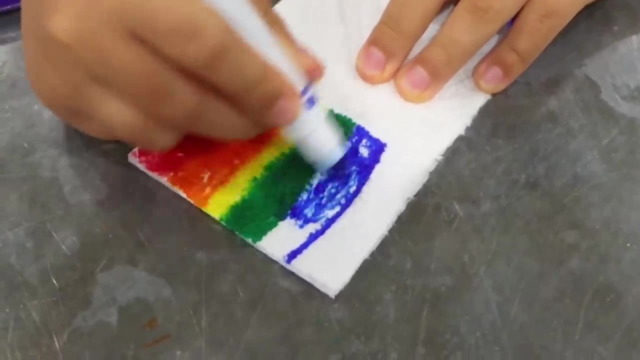 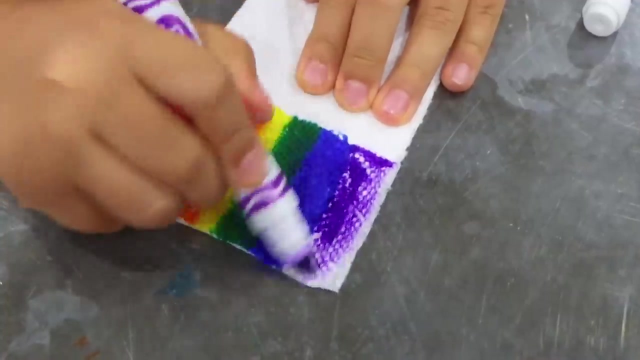 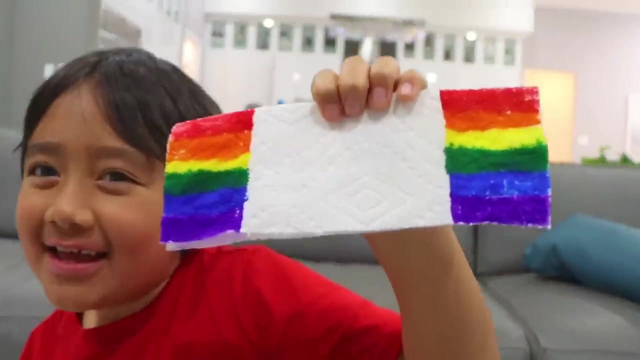 Next is green. Fill it in Green. Next up is blue. We're going to finish it up with my favorite color, purple. Now do the same thing to the other side, like this, See, Like. so Next, fill up your two thingies of water. 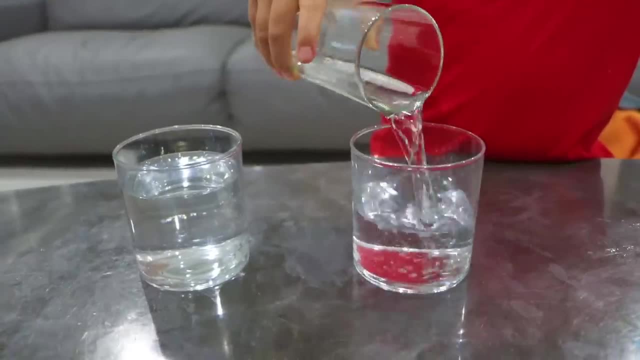 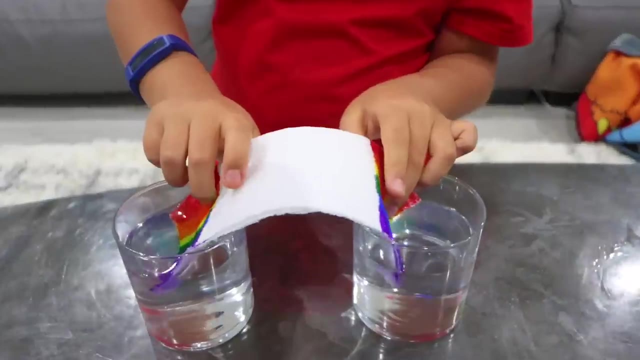 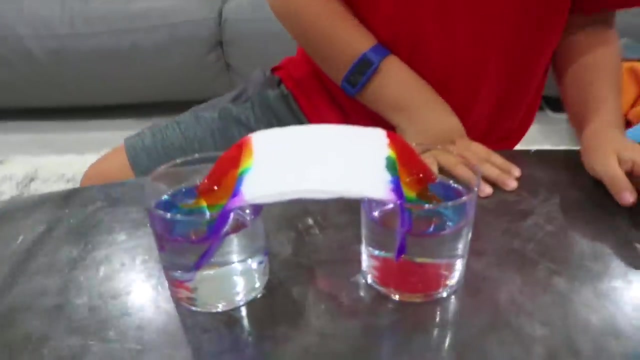 And the second one. Now take your rainbow paper that you drew and put half of both of the sides in the water. Now we wait. Watch the rainbow form. It's already forming a little bit. Whoa, guys, Did you see? 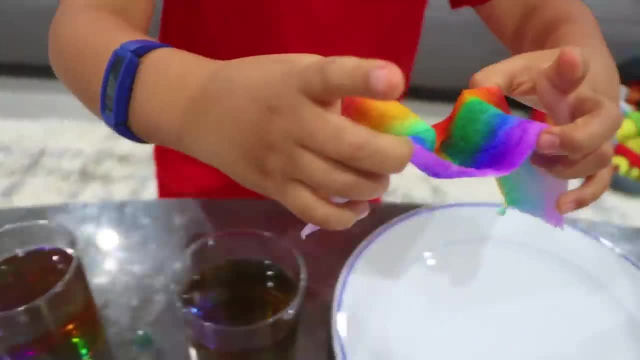 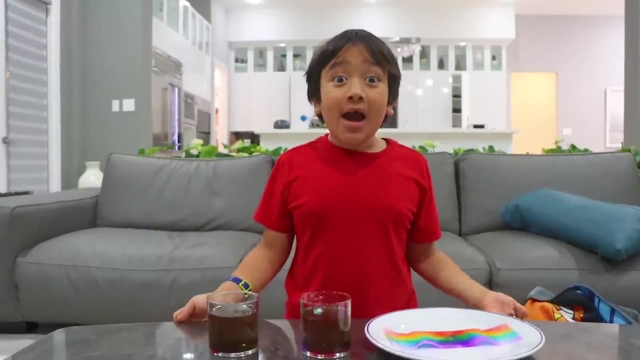 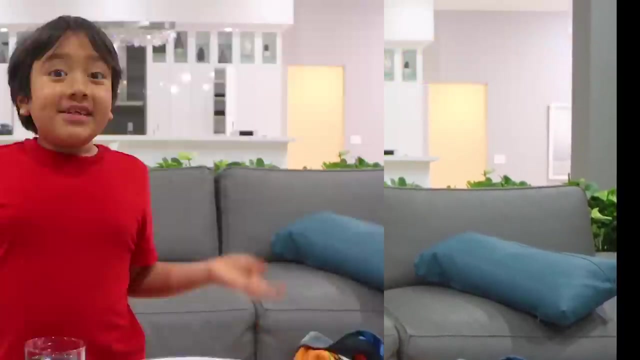 We made our own rainbow. Whoa, Put it right here. This is so cool. Did you see the marker die? move up the paper towel and touch each other, Because that's called capillary action. Did you know regular plants also use capillary action? 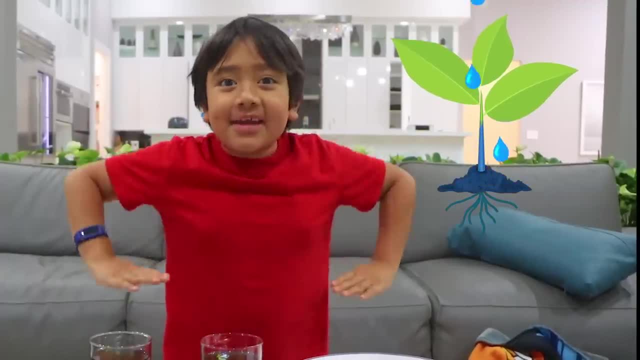 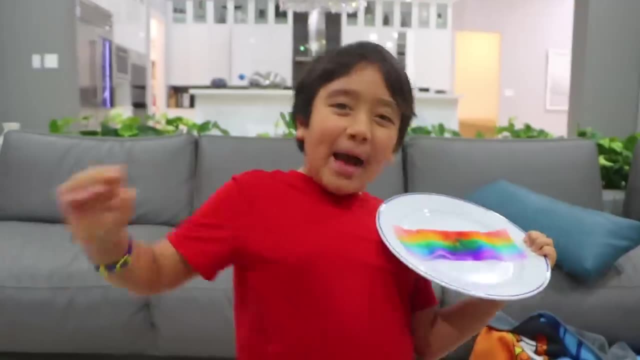 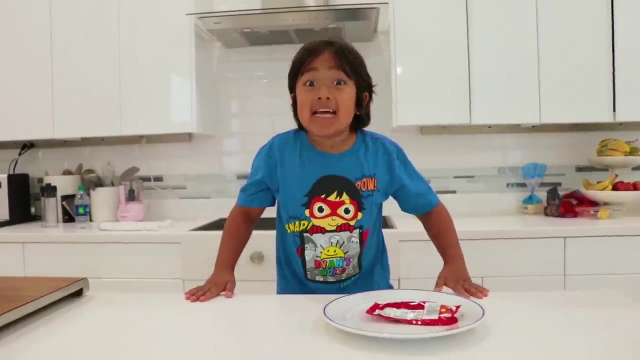 Because they bring the water from the roots and make it go all to the other parts of the plants. I hope you guys had fun making our own rainbow together. Bye, Remember. always stay happy and rise up. Bye, Hi guys. Today we're doing a science experiment with Skittles. 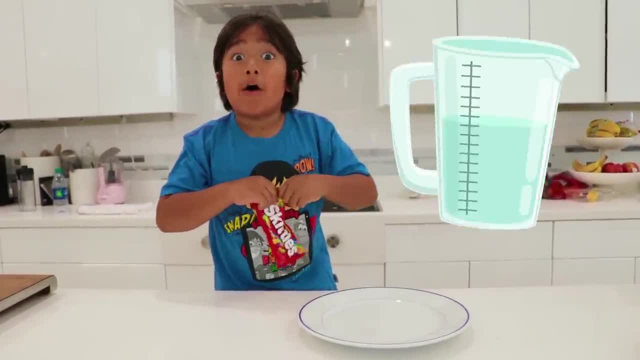 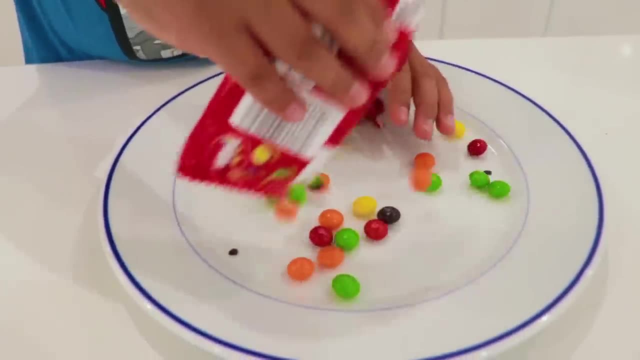 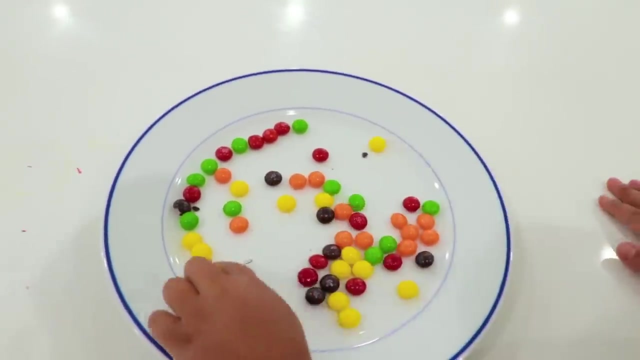 We're going to see if Skittles' color dissolves in water, and I think it does. Whoa, Whoa. Now we're going to spread the Skittles around like a circle on the plate. I'm spreading all the different colors around like this. 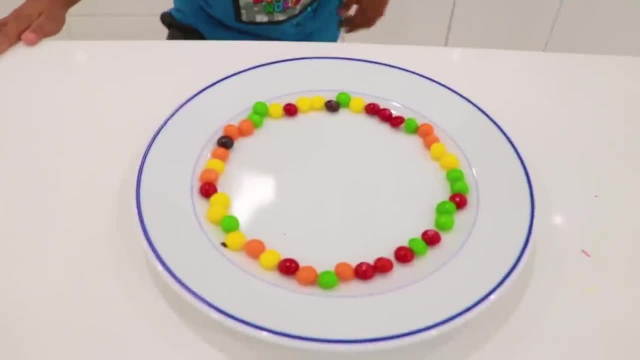 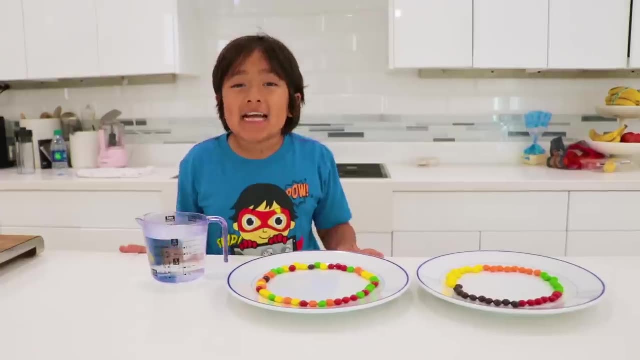 All done. Look, You can do it however you like, because I made it like this and like this. These are all the colors together. Next, let's pour water onto the plate. Ryan's using warm water, Okay, So don't forget to ask a parent for help. 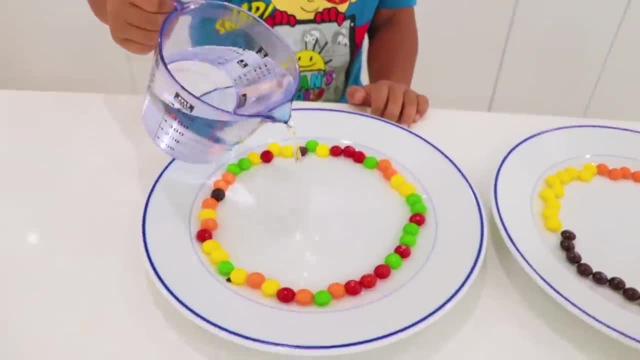 Now we're going to see what happens. It's already happening. Whoa, Look what's happening. So cool. So the more they are together, the more bigger they are. So what you notice is that the color is beating in the middle right. 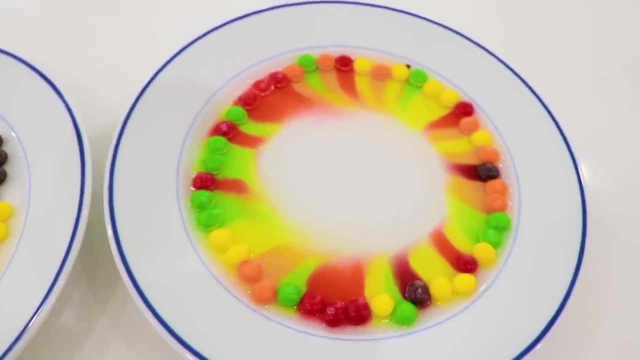 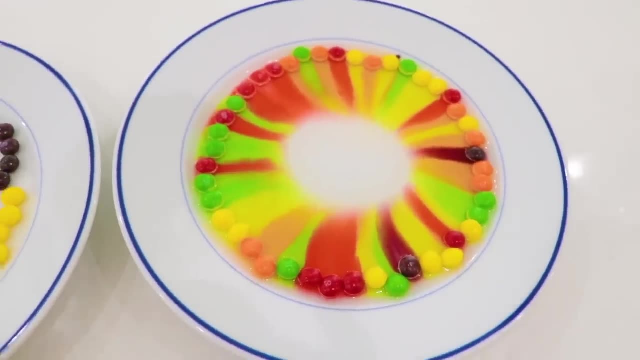 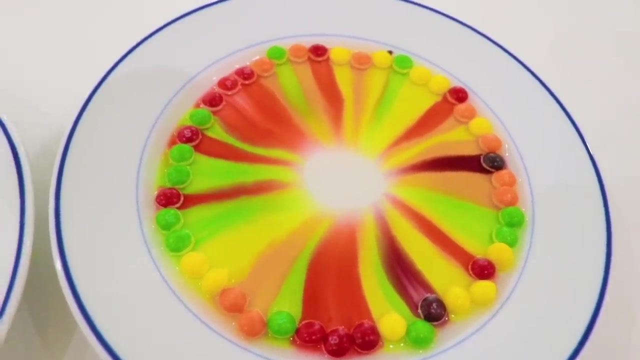 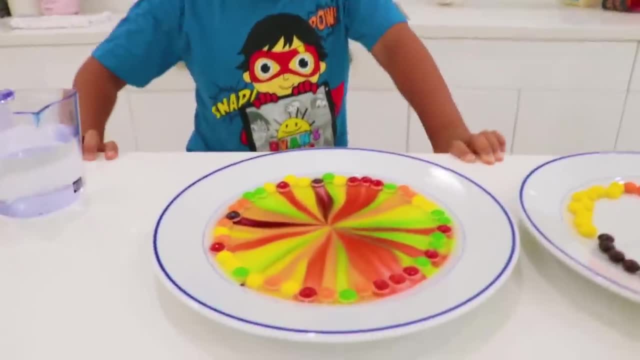 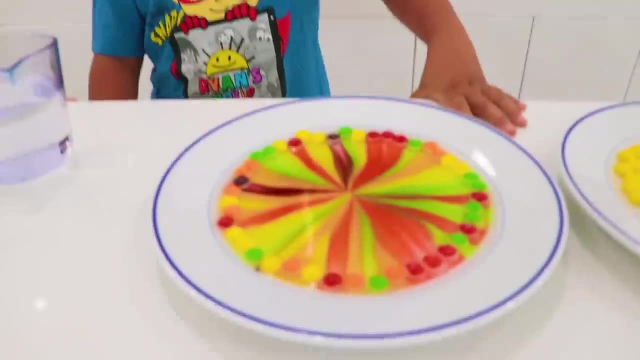 Oh, Just like that, Okay. So what's that do? Huh, Whoah, That's so cool. And what did you notice? Did the color mix together? No, look it separated Right. Yeah, All of their colors did not mix. 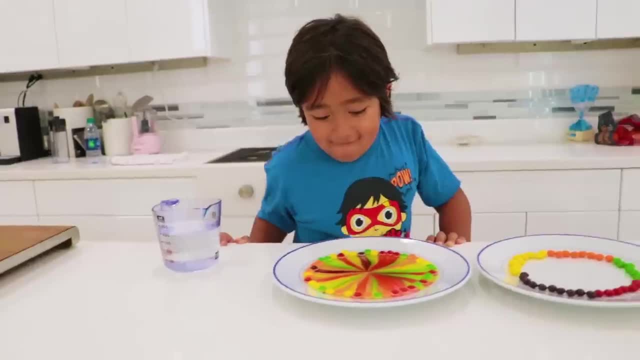 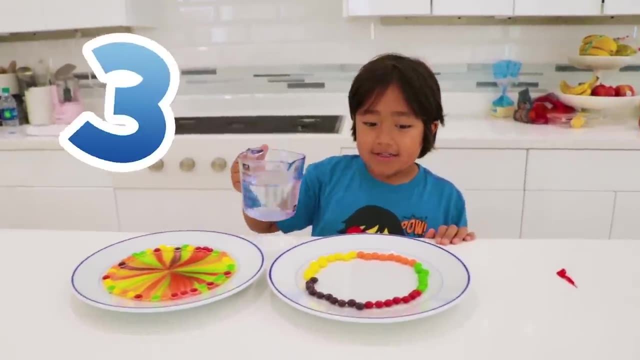 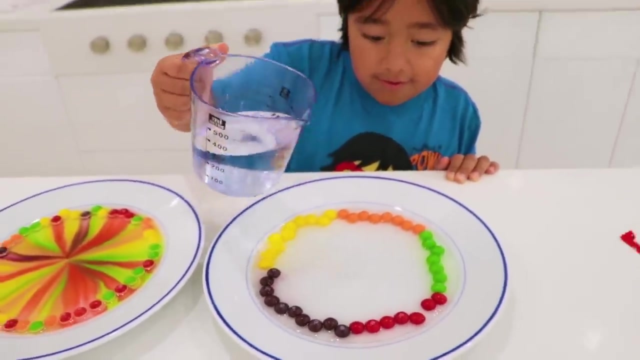 Only meet in the middle. Now let's try the other one and see what it looks like. I think it's going to. those colors are going to be really really big. Three, two, one, Yes, Yes, Oh, What's happening? 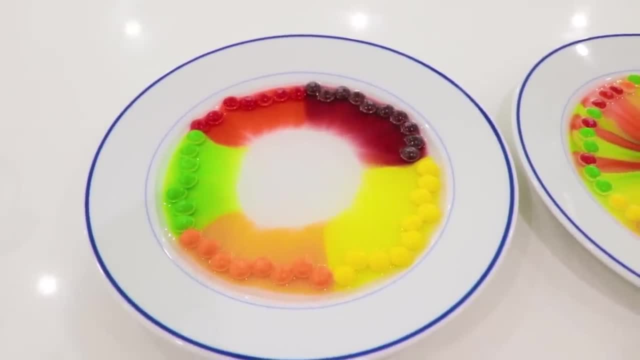 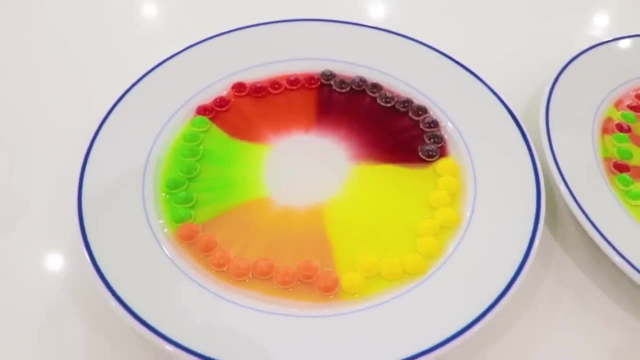 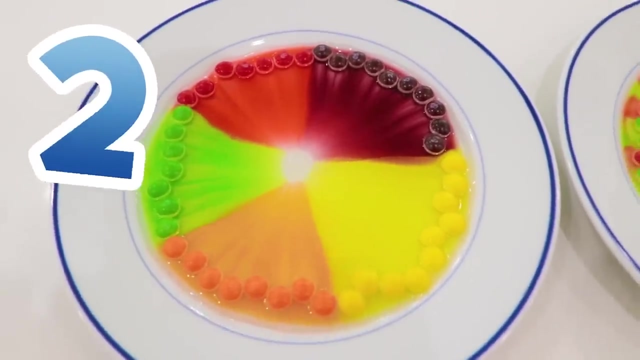 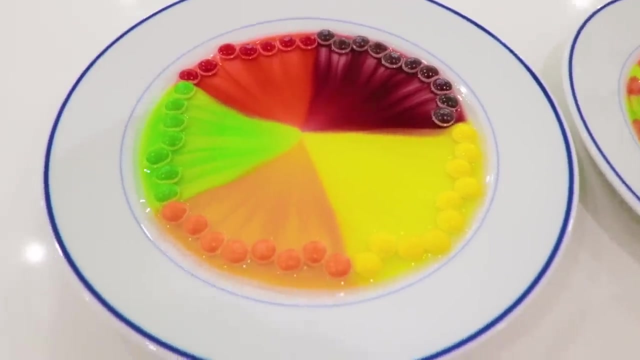 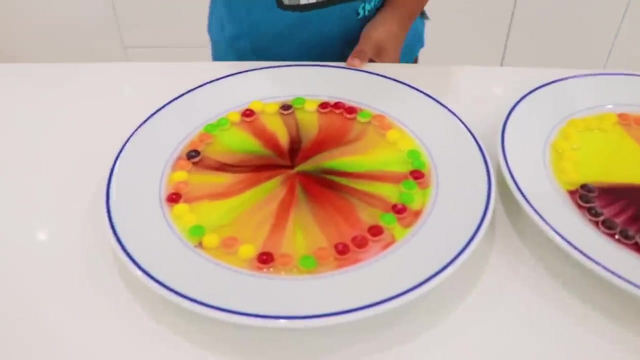 No, you know, there's like a little Toy thingy versus this car, this car, and you have to follow it. It kind of looks like that: Oh yeah, it does. Three, two, It looks so cool, guys, it does. and look, since we did different patterns. 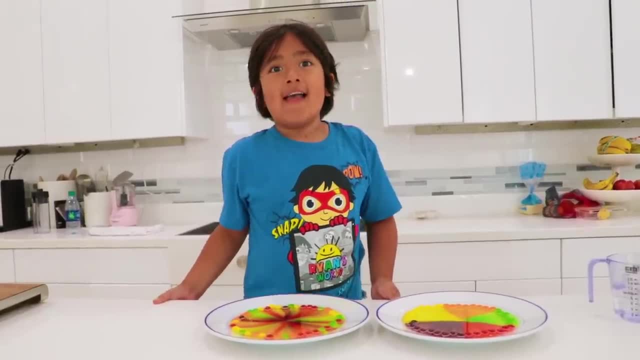 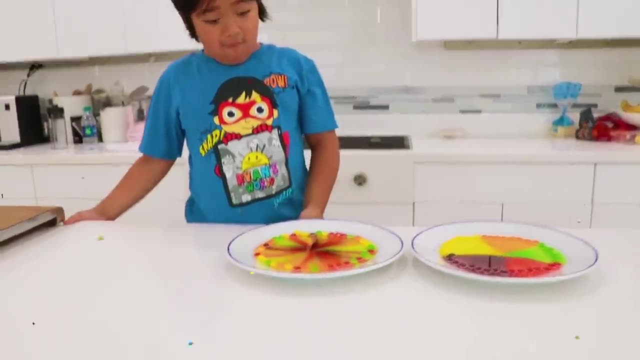 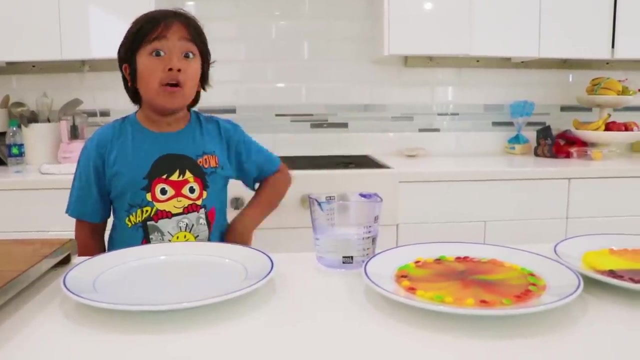 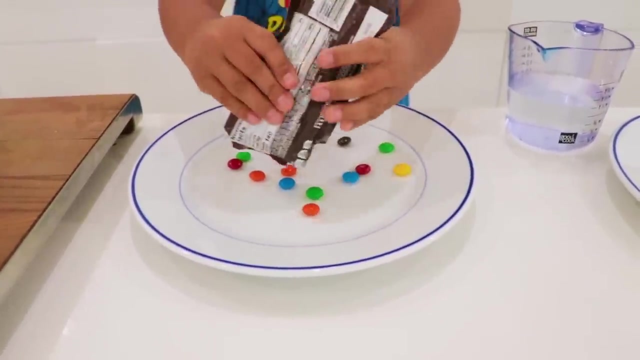 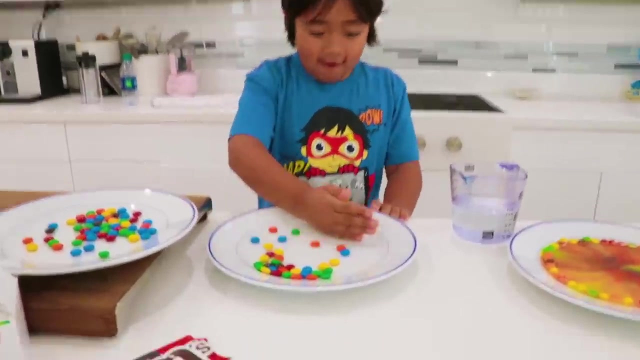 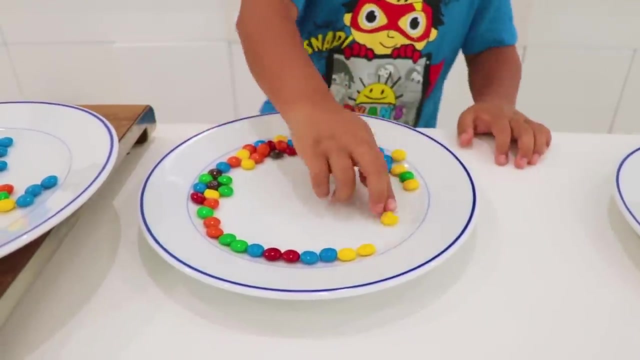 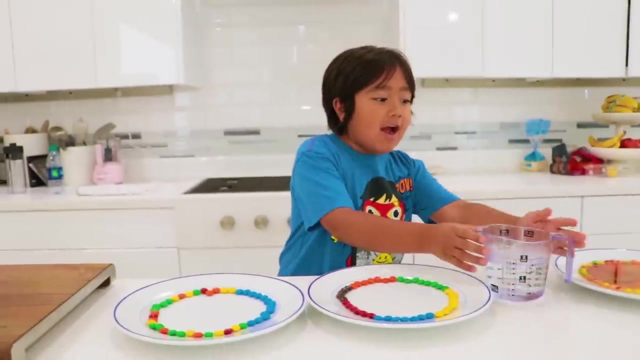 They look differently. The question was: did the skittle colors dissolve in water? Yeah, food coloring on the skittles and the sugar, both dissolving water, Dissolving water. find out Now. spread them out on the plate. Now I have two of them again. I have one with a lot of colors and I have one that's random. Let's try. 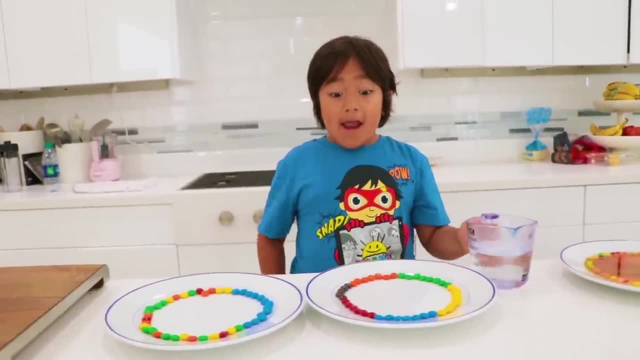 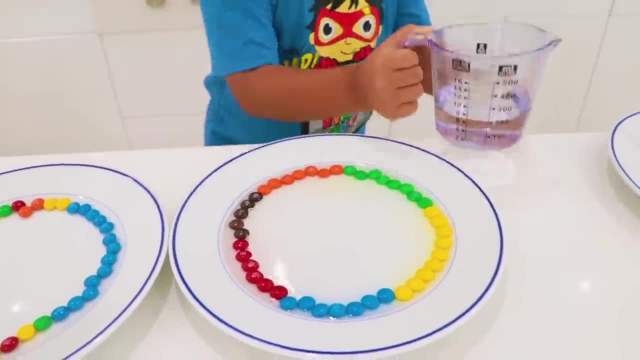 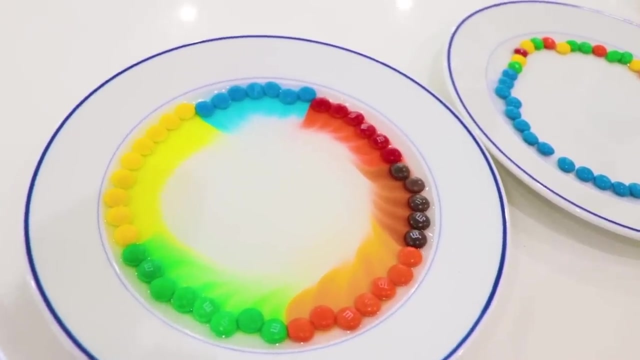 But we're also using warm water, So we're gonna try one with warm water and one with cold water. Let's see if it makes a difference. Warm water, right here Starting: Is it working? Yeah, it is, Whoa. So this is the M&M's. 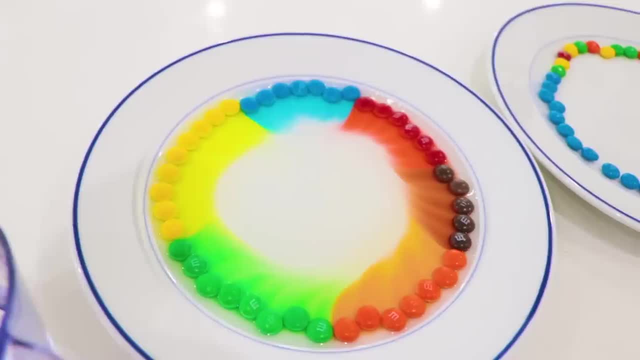 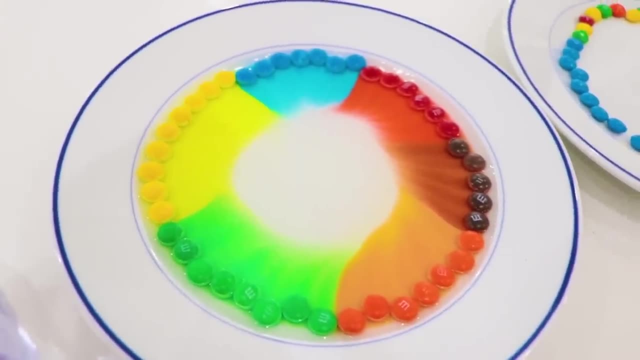 Do you guys see any difference between the M&M's and Skittles? Yeah, the M&M's like twist. It looks so cool, Aww. So you feel like it's the same speed or you feel like it's different speed. 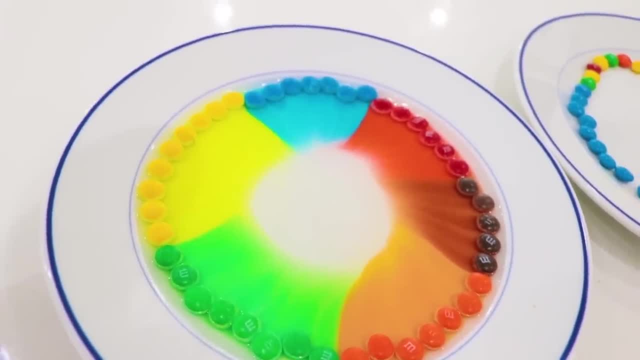 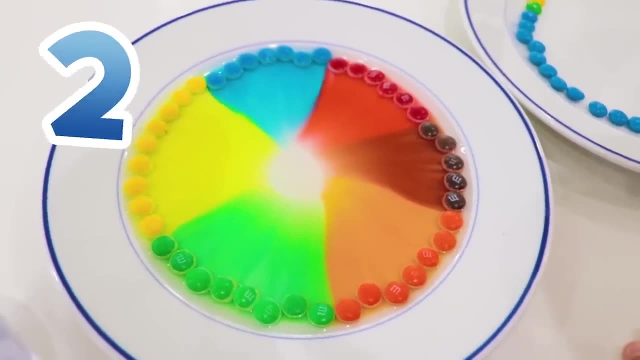 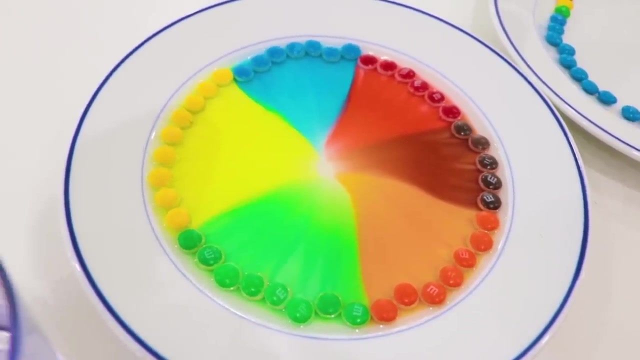 It's different speed, So you think it was going slower than the Skittles, or faster than the Skittles, I think faster than the Skittles. Three, Two, One, Bye, bye. There you go, guys. M&M's. 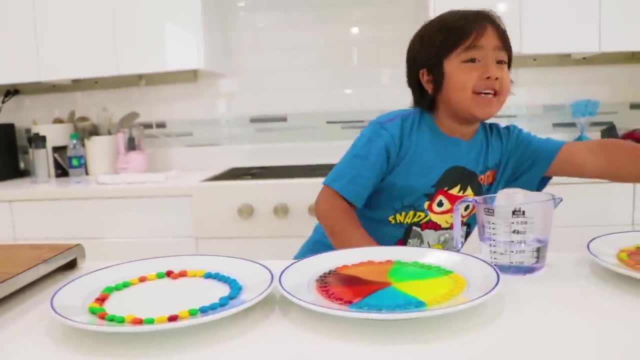 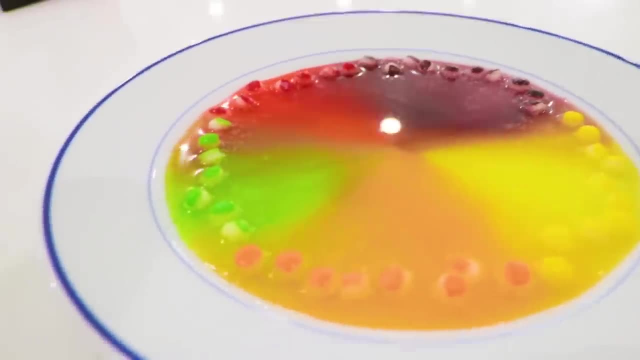 Which one do you like better, the M&M's or the Skittle one? So we've been letting these sit out for a while, so it looks super different. Everything is coming together There And here. if you guys look, it's all the little M&M pieces on the back. 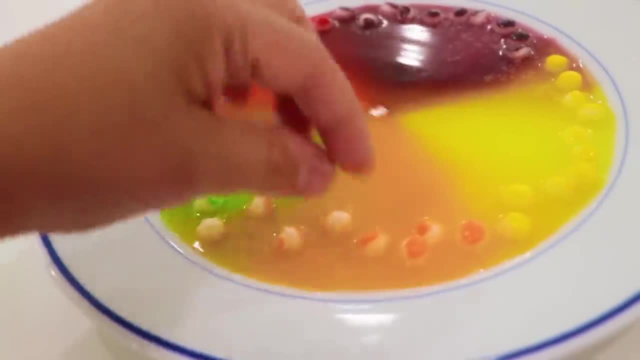 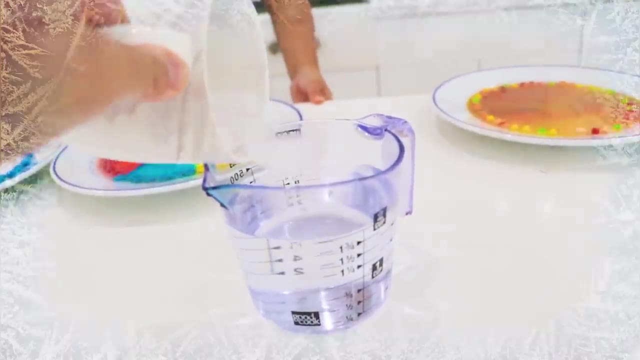 It's all white now. So instead of the color, they're all white, Do you see, Because all the colors are coming out? We got regular water for the sink and now we're going to add ice to it to make it ice cold. 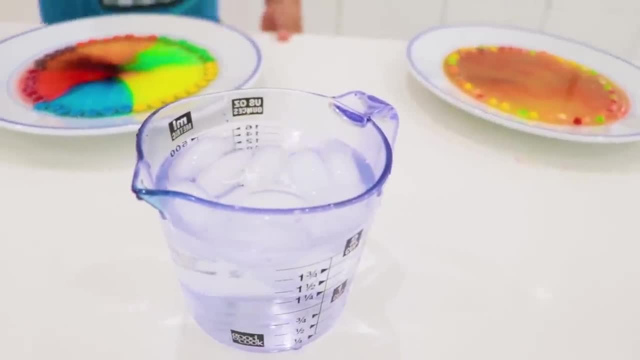 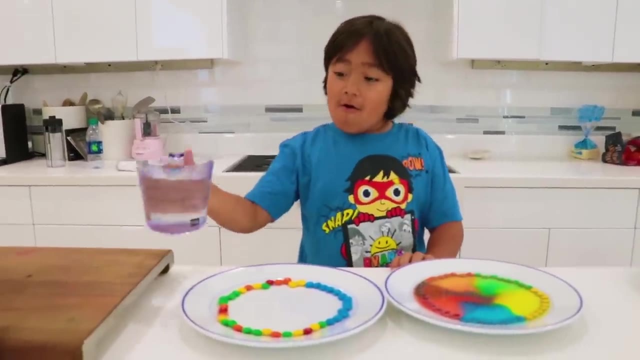 Ooh, We're going to let it wait for like one minute. That's right, Ryan, to make the water cold. Yeah, Okay, I think it's ice cold now. Oh, Three, Two, One, Two, Three, One. 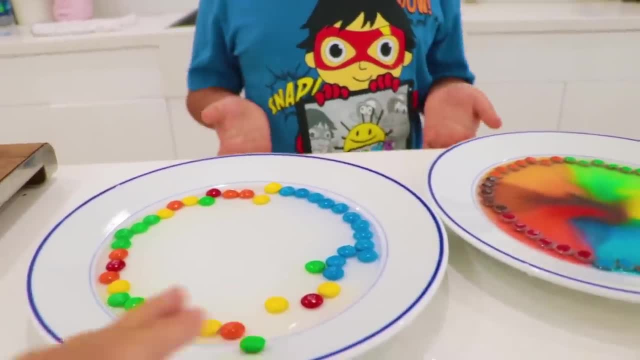 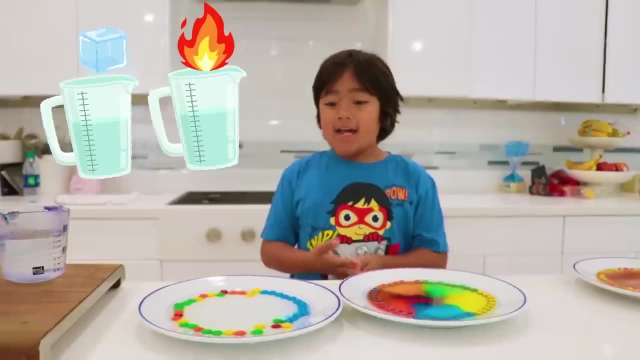 Two One, Two, Two One. I think it's going to dissolve. No, Oh, While we wait, do you guys think it's going to dissolve? Good question, Ryan. What do you think? Do you think the cold water or the hot water will help it dissolve faster? 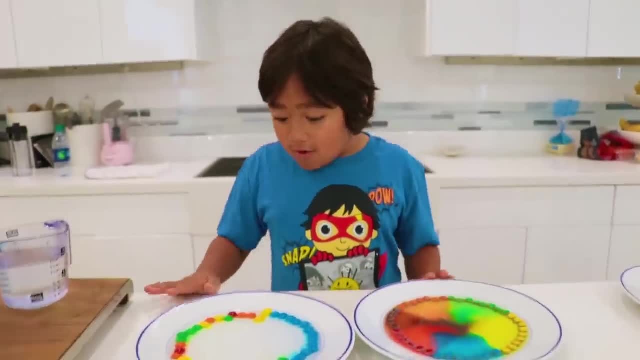 I think the hot water will dissolve faster. Okay, let's check it out and see Whoa. We're going to have to wait. It's working. Oh, if you move it, it goes faster. We're going to wait and see what happens. 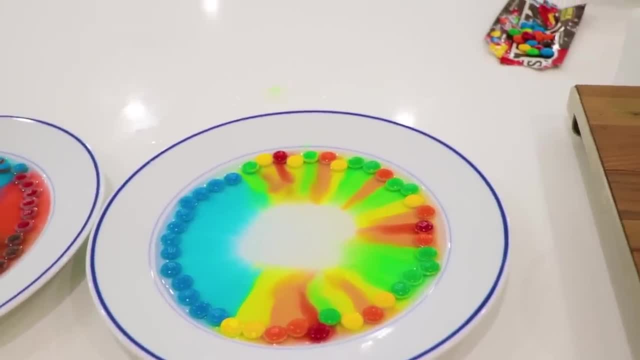 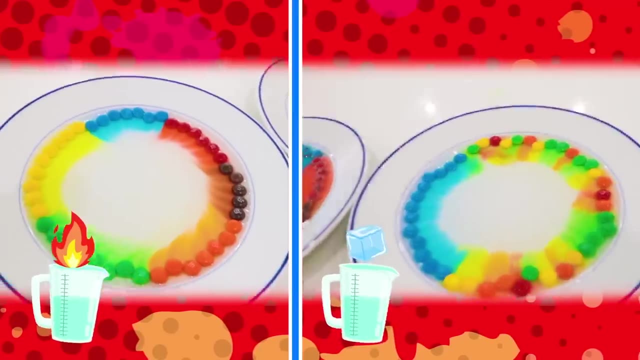 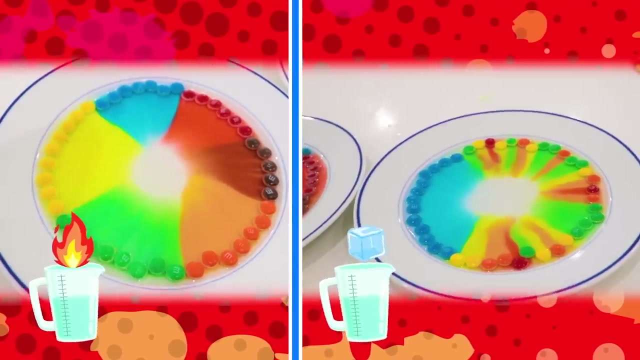 So there's the cold water. As you notice, I think it's going a lot slower. Yeah, Is it going to dissolve? No, yeah, we're waiting for a while now. it's still working. yeah, it's just not going as fast. wait, we're waiting. what happens? if you like, blow it. 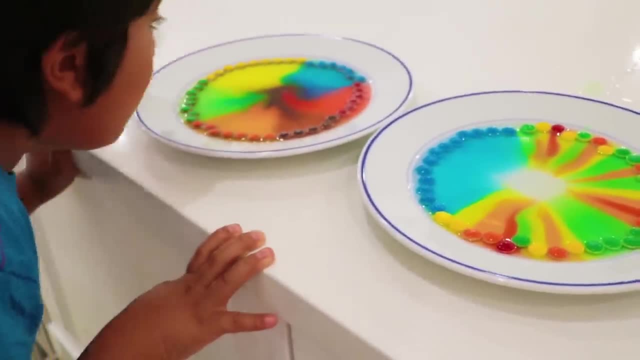 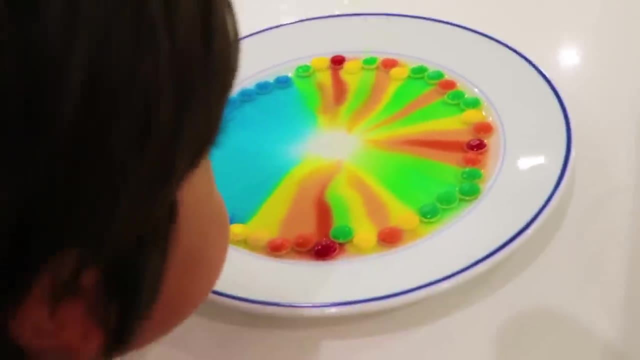 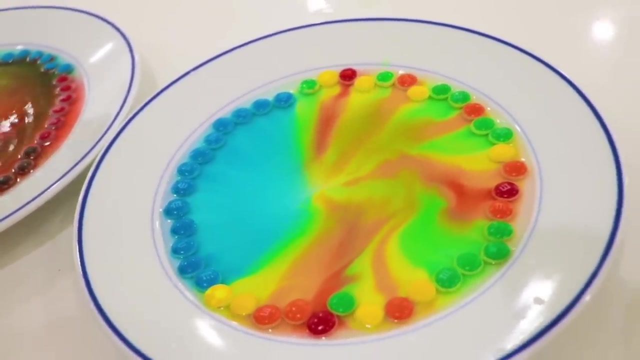 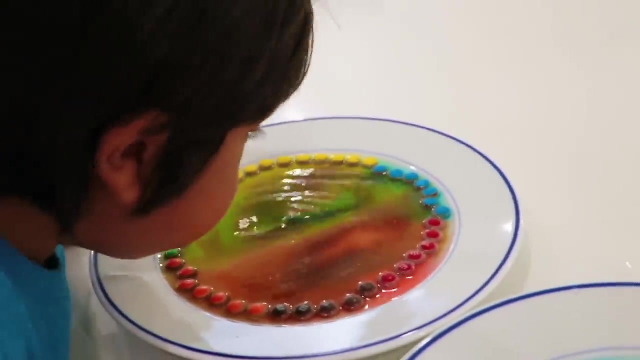 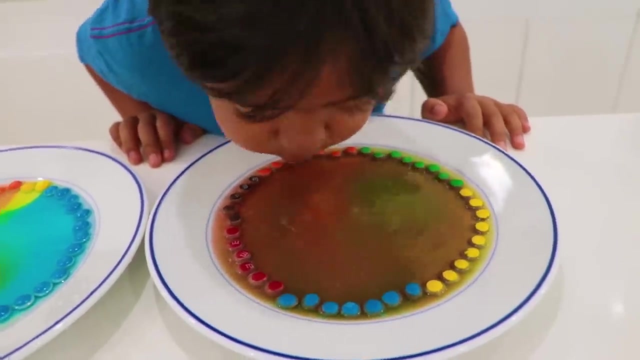 oh, my question, why don't you do it? oh, it doesn't change it, just change the water. so this is still going. wow, it's mixing it all together. whoa, it's creating like a galaxy color. wow, that looks cool. oh, the other one looks cool. when you mix, you can try to blow that one too. 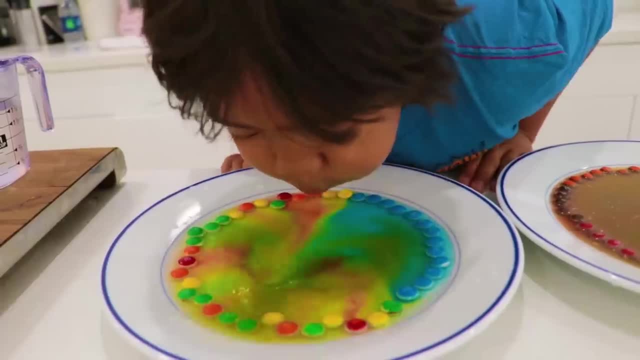 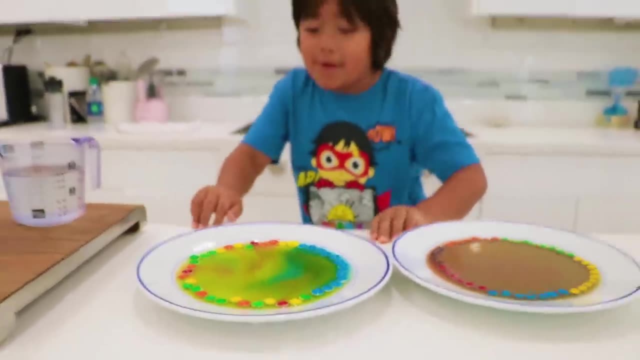 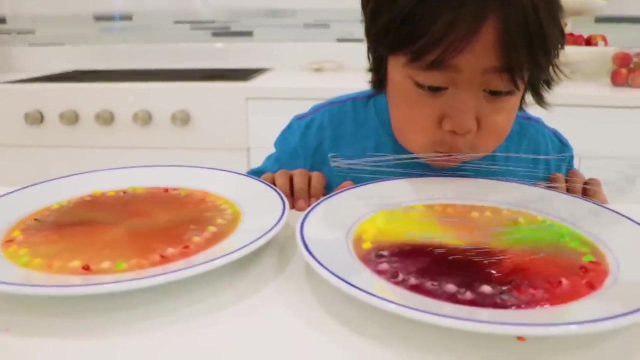 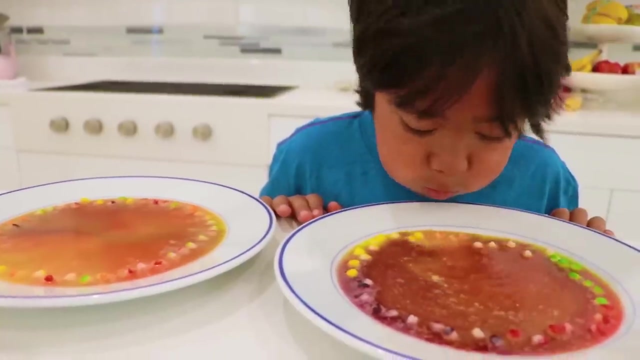 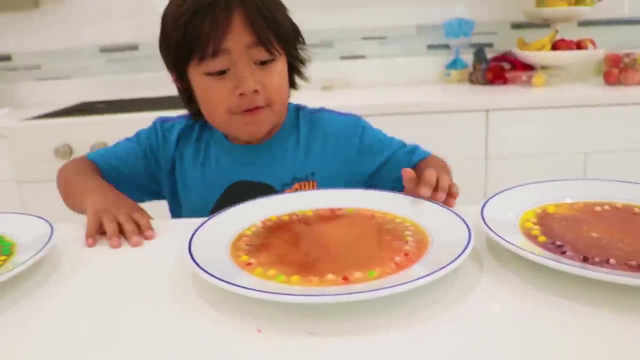 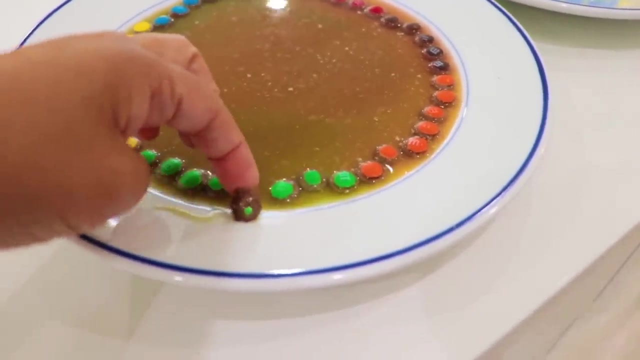 it's. it's like a tornado when i blow it. i know so ryan's trying to mixing one color. oh, this is turning during. convince me, this is the m m's here. so it's because it's chocolate. when the color dissolves, you see the chocolate left over, right, yeah? 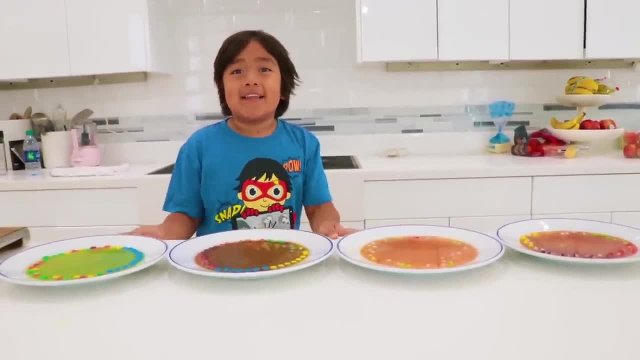 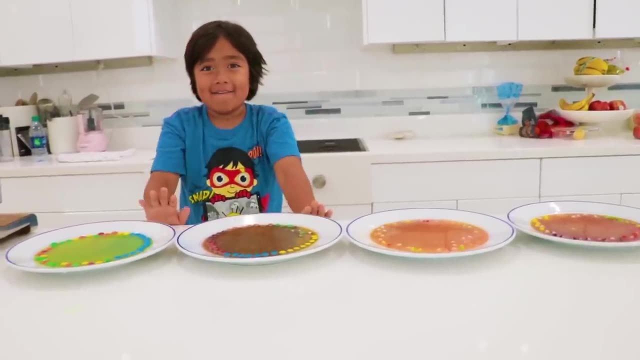 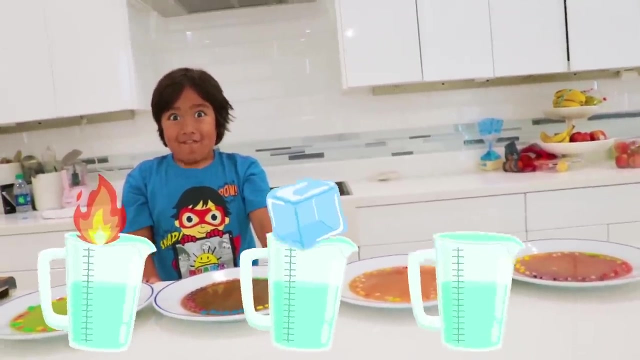 thank you so much for watching my video. if you liked it, then like and subscribe. bye, remember, always stay happy and rise up. bye, bye, guys. then you guys can go out there and do your own science experiments right, trying hot water versus cold water versus warm water, trying Skittles versus M&M's. 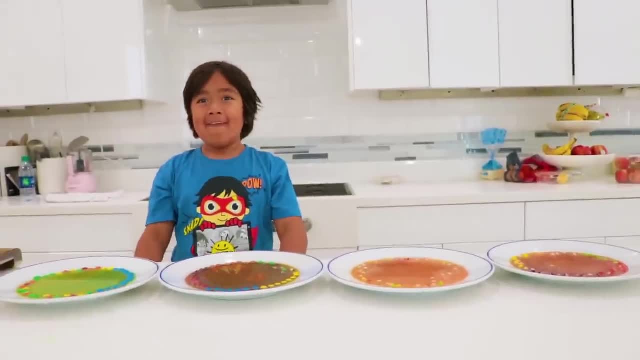 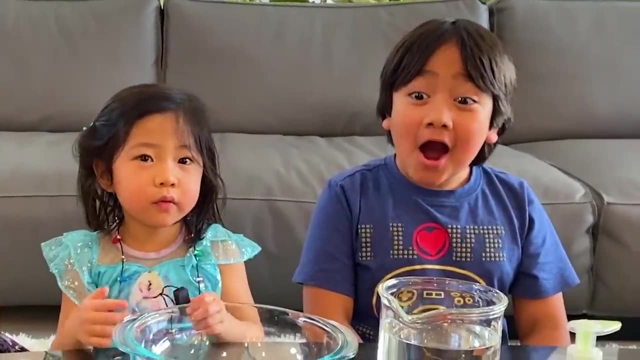 and maybe there's other candies we haven't even thought of. So much fun. thank you for watching Guys. today we're gonna learn how important it is to wash your hands. Yeah, so you know how long you're supposed to wash your hands for. 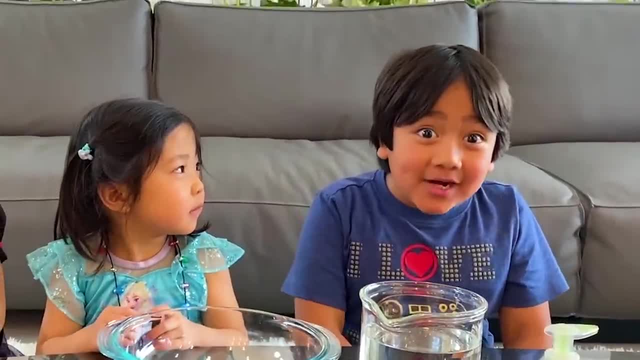 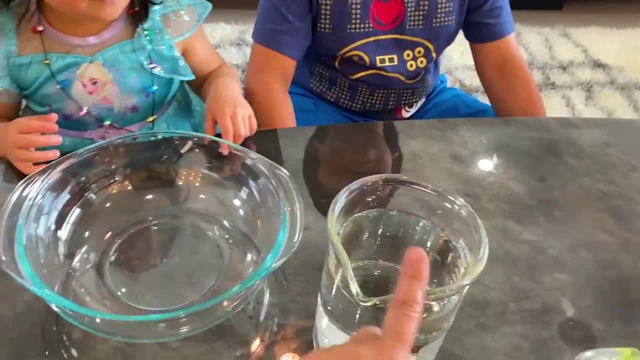 Yeah, How long You're supposed to sing happy birthday two times? That's right, so it's about 20 seconds at least, okay. So here's the experiment I want you to do. This is water. pour the water in there, okay. 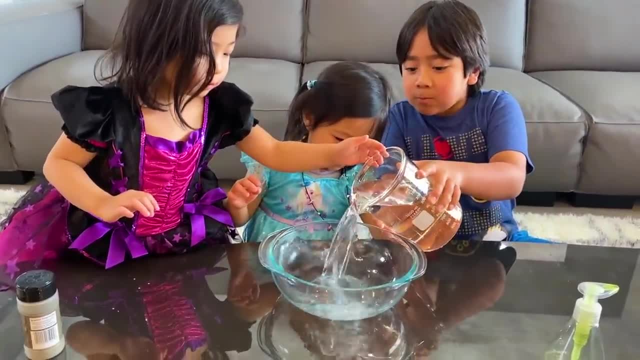 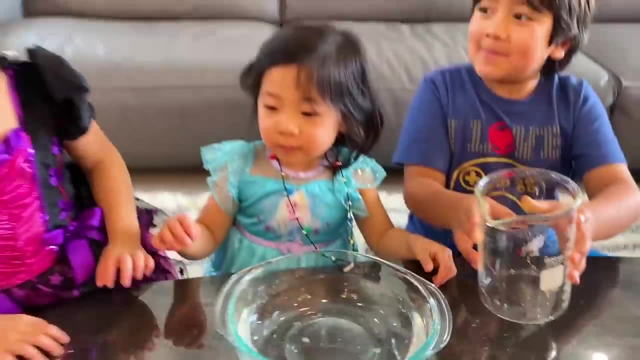 Do it very, very carefully. The whole thing, The whole thing. yeah, Yeah, I helped Brian, You did help Brian. So this is pepper. any pepper you guys have, this is the one that I have in the house, okay, 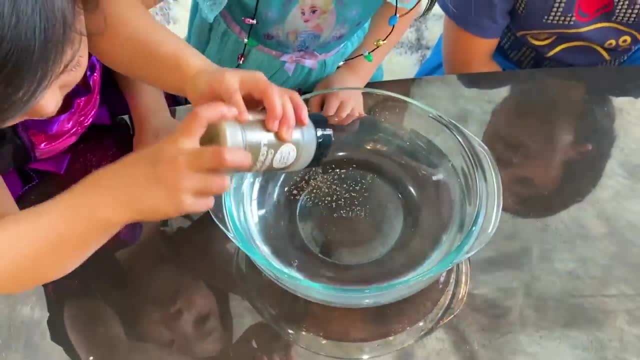 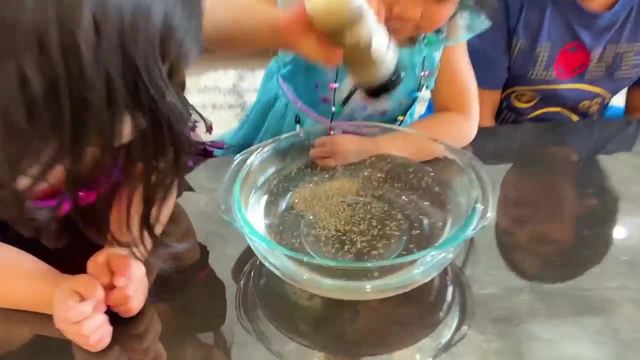 So sprinkle some peppers in there. Do I wanna do it? Yeah, take turns, Sprinkle more. You can do a lot more than that. There you go. That's a lot. Next step is: I want you to take your little finger. 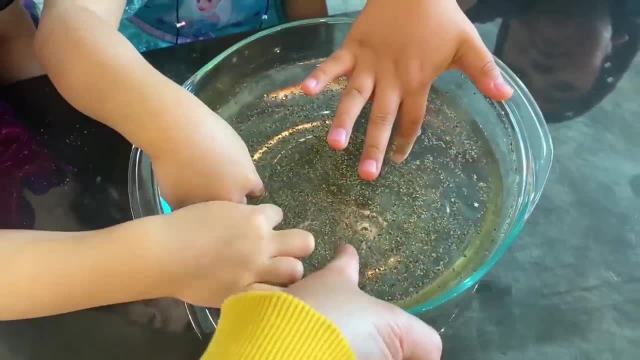 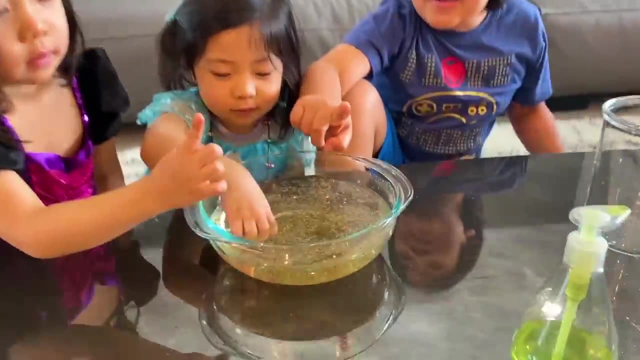 and dip it into the pepper water. Now I want you to pretend these pepper water are germs. What happens when you take your hands out? Oh no, there's germs. Yeah, you see. And if you touch it, there's germs, right. 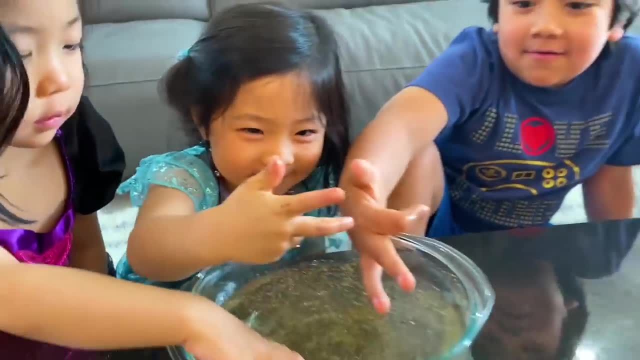 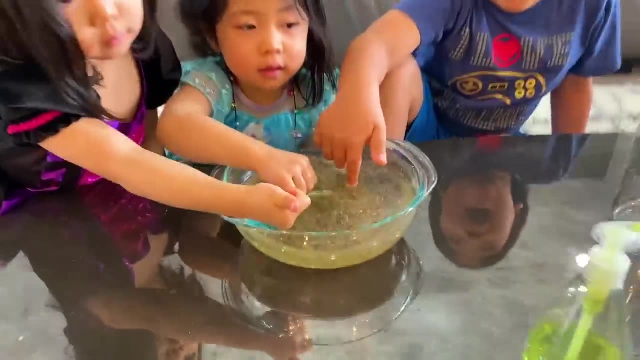 Look, oh, there's germs on you. There's germs on me, I know You see the germs, Yeah, Okay. So here's why it's important to wash your hands. You ready? Yeah, Okay. so that's what happened without soap. 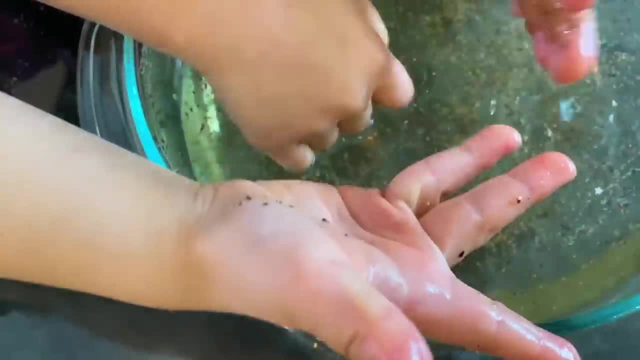 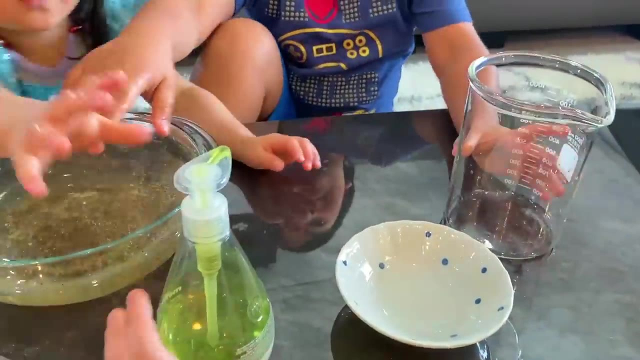 It just sticks on your hand right. Ooh, germs everywhere. Ah, Next, I want you to squirt soap into here. I wanna do it. There you go. Can you squirt some soap into there? I hold for you. 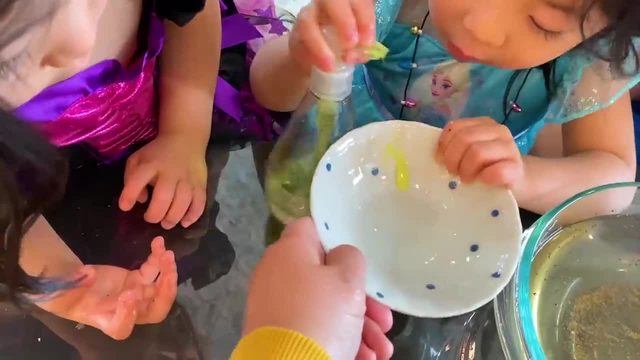 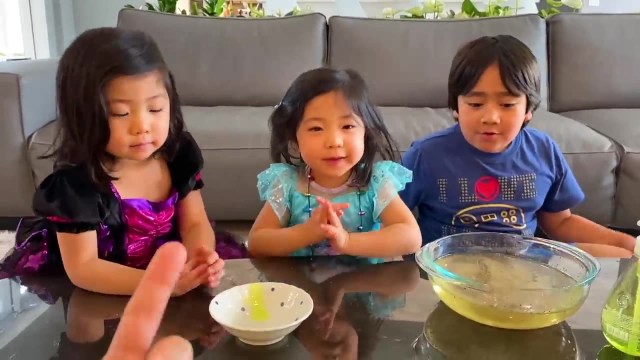 Whoa, There you go. good, All right, okay. turn, There you go- all right, Okay, that's a lot. Here's what I want you to do: Take your little finger and then dip it into soap. 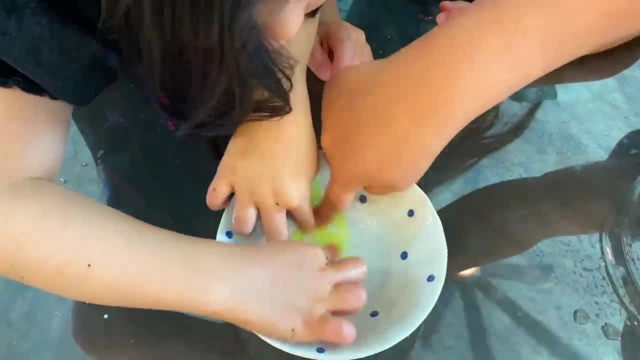 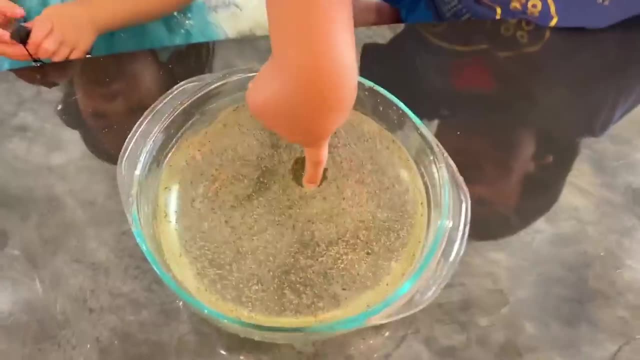 There you go, dip in a lot, Okay. so this is why soap is important. First, Ryan's gonna do it. Okay, go ahead. Whoa, What happened? The pepper's going away from the soap. I know it looks like the pepper's running away. 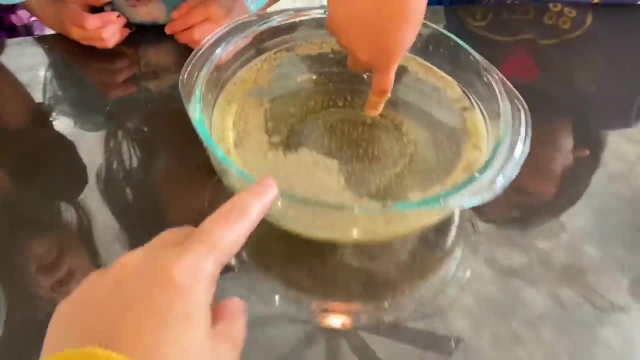 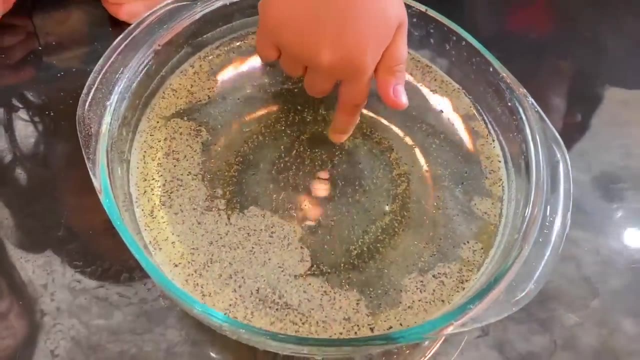 from the soap, right, Yeah, So think about it. So if these are like germs and bacteria, when you put your hands in soap and wash your hands right, all the germs and bacteria are no longer on your hands. 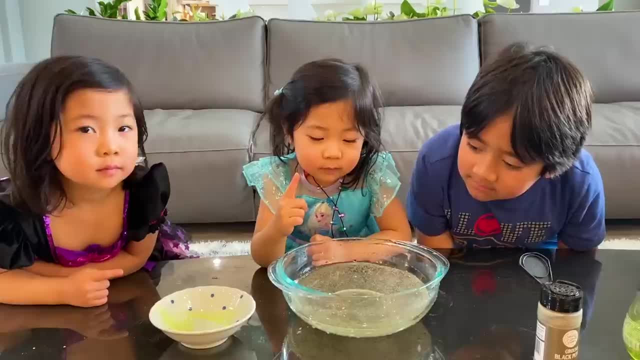 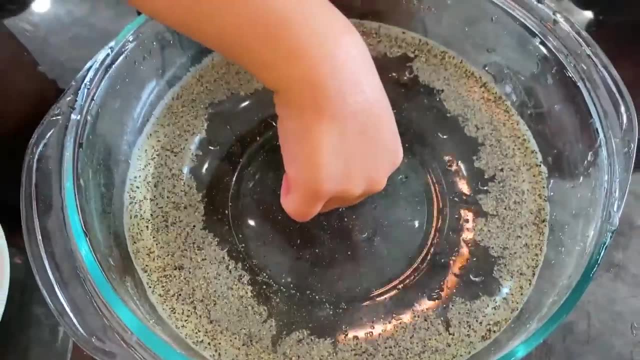 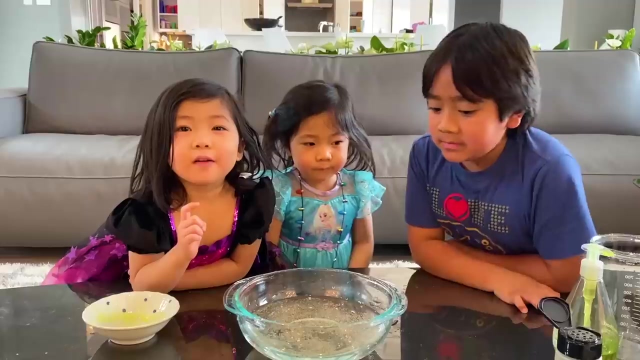 Yeah, They're running away. Can I try? Yeah, of course It's my turn. Okay, Whoa, that's so cool. See how it's running away. Whoa, That's so cool. Whoa, All right, Kate, you wanna try now? 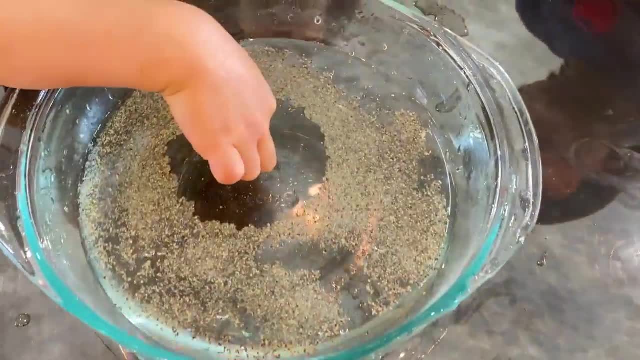 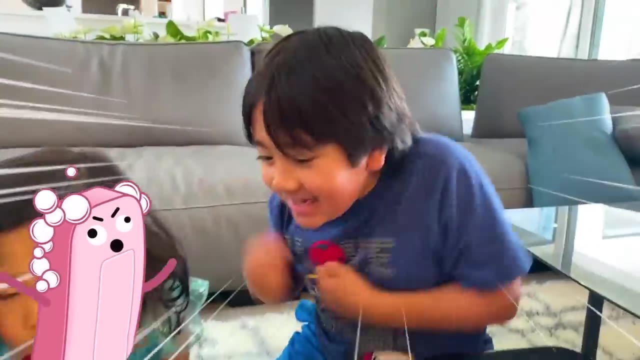 Okay, guys, it's my turn. Whoa, it's running away too. Yeah, Isn't that cool. Yeah, It's like: oh, no soap. Ah, That's why it's very important to wash your hands. 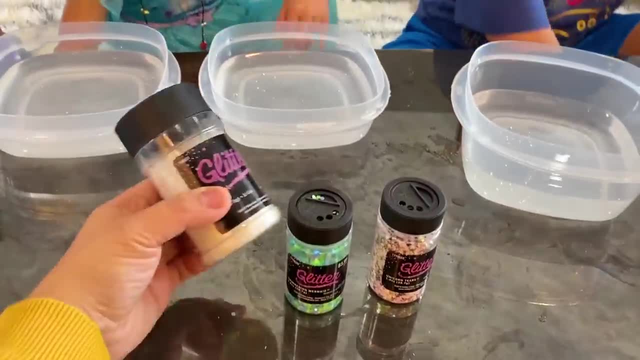 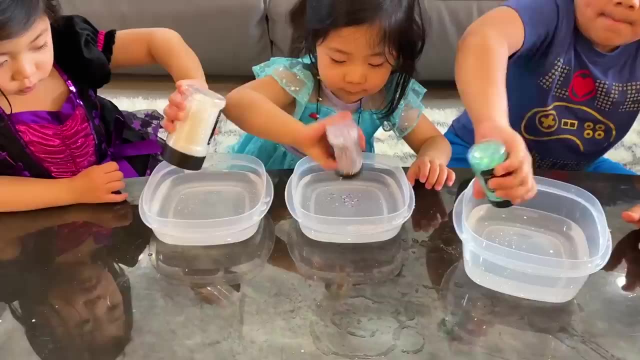 Now we're gonna do it with glitter, Yeah, so you guys can each take a glitter or a share. I want this glitter And put it into water and pretend these are germs. There you go. I'm putting a lot, You're putting a lot of germs. 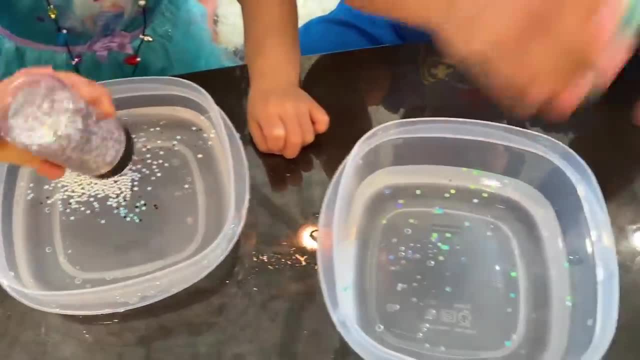 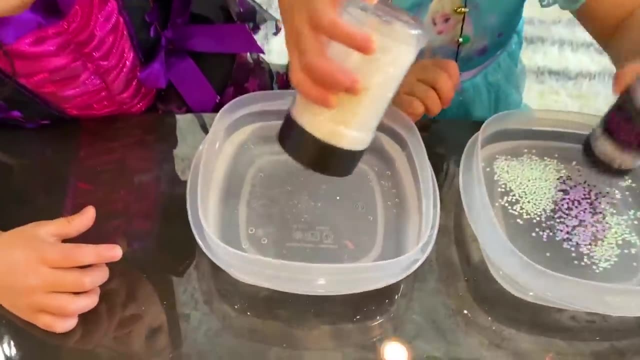 Yeah, I'm gonna put a little bit, Okay, a lot of germs for Emma. There you go More, And then we can all share: Ooh cool, Kate, There you go, I'm adding some white germs now. 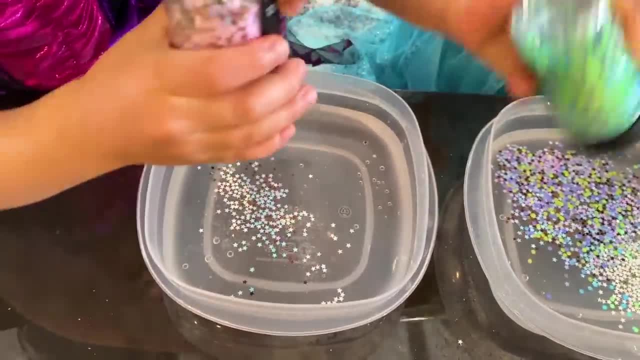 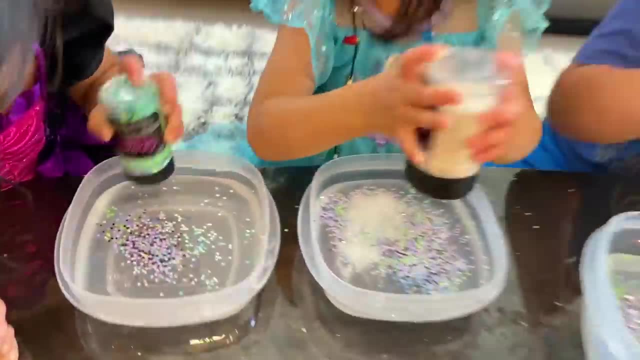 Yeah, I want some white germs, Different types of germs. Yeah, Shake, shake, shake, Shake, shake, shake, Shake the glitter. I mean shake the germs. I'm shaking the germs, Ah, germs. 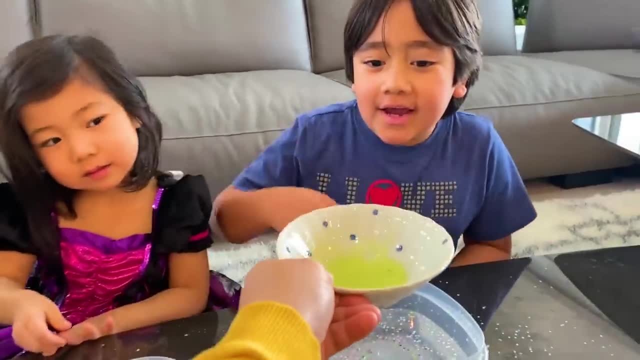 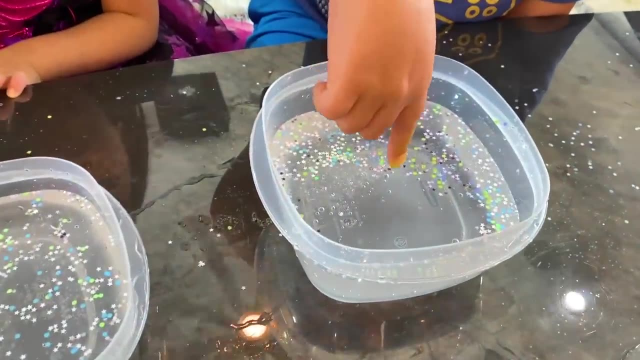 Yeah, Good, Now let's try the power of the soap. Okay, Okay, put the soap on, Okay, And then put it in. Wait, it's going away. Yeah, it's moving away from your finger. Yeah, it's like wah. 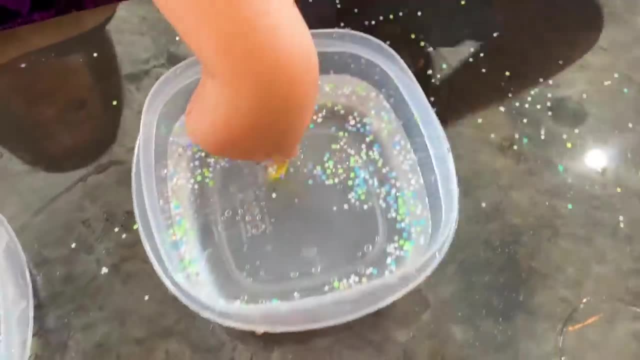 There was one right here and it was like poof. Yeah, All right, Kate, your turn. It's yours, Dip it in there. We're gonna use quite a lot of soap. There you go. Good job, girl. 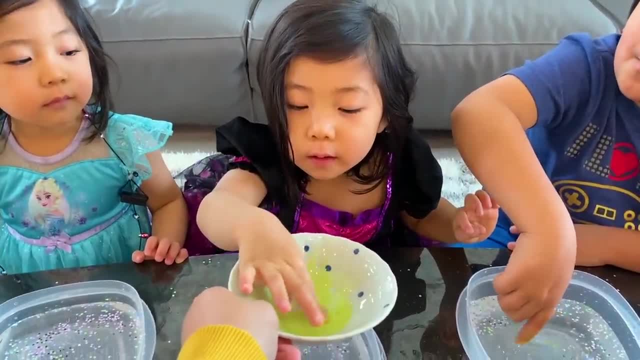 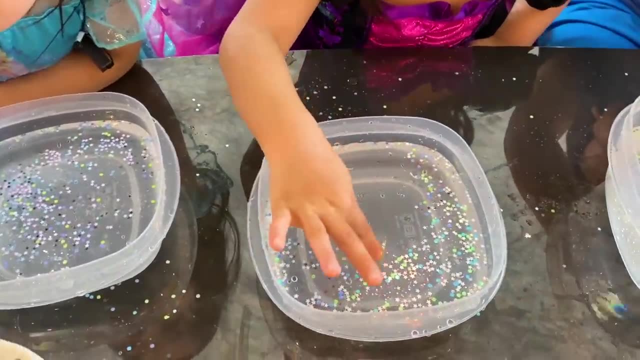 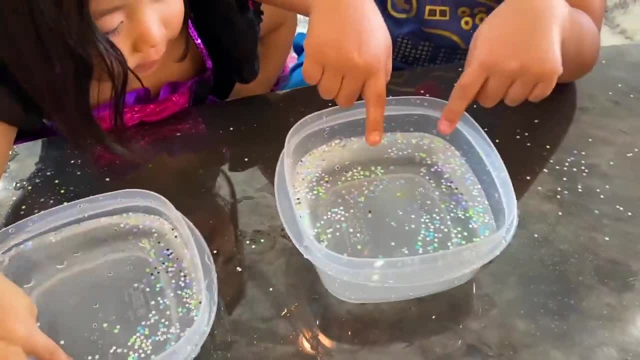 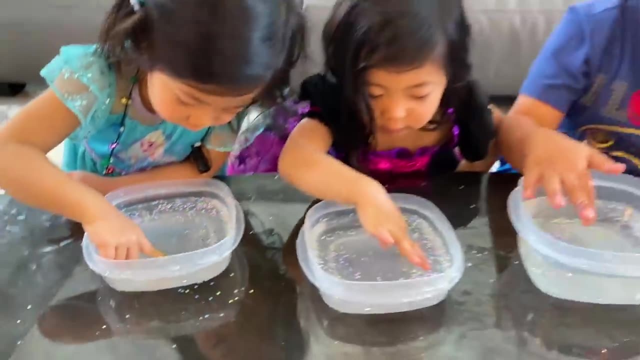 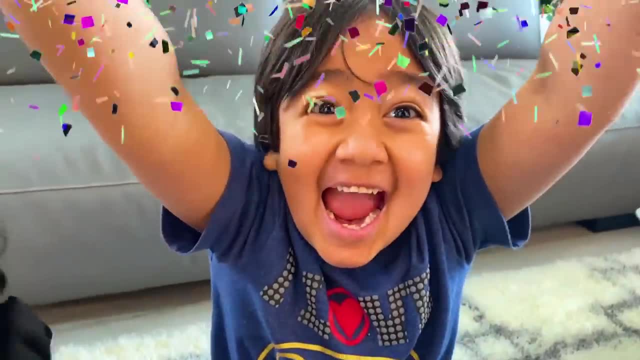 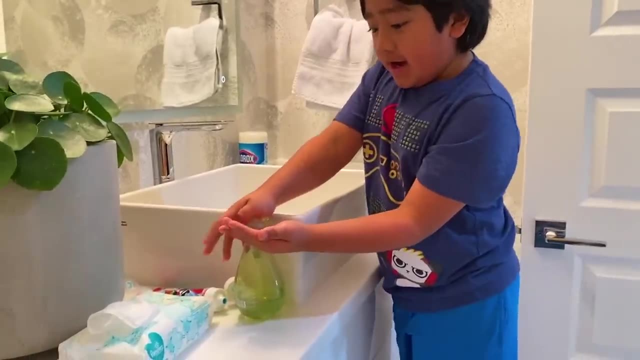 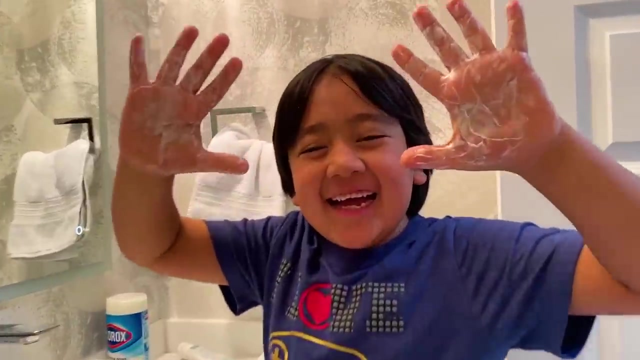 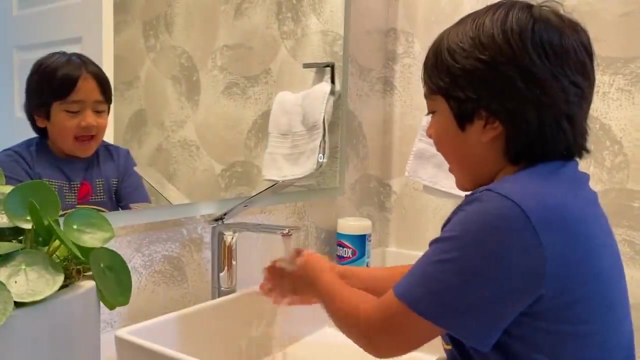 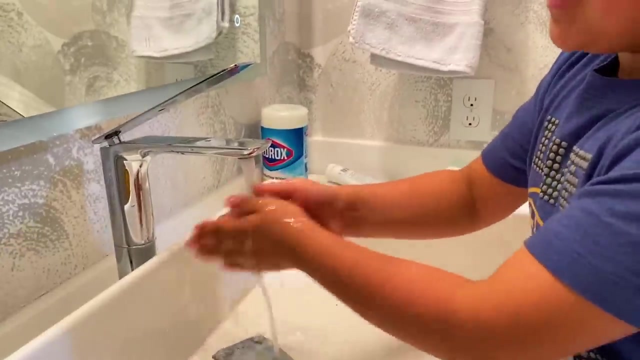 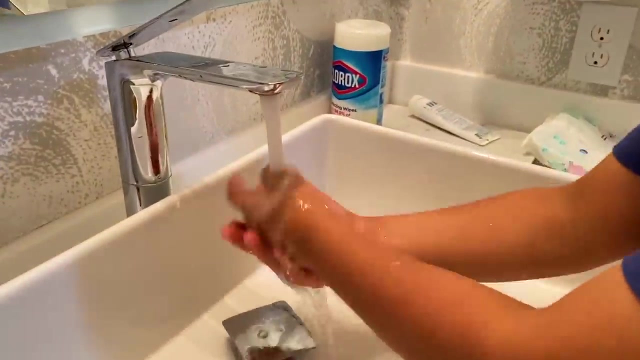 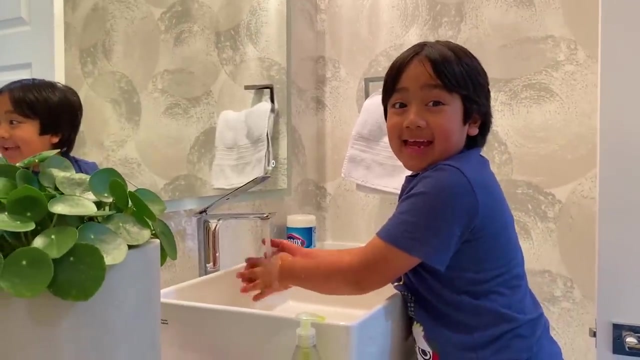 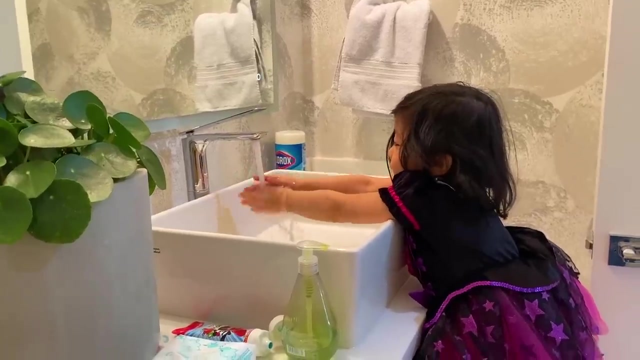 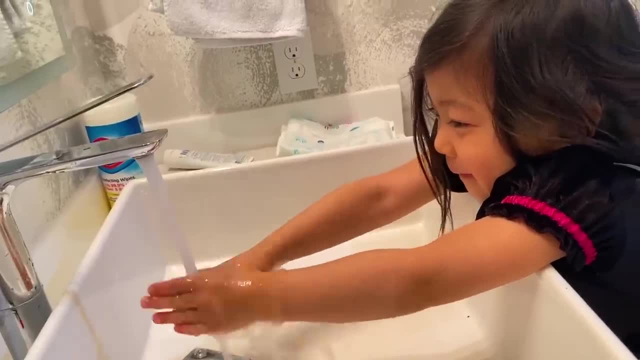 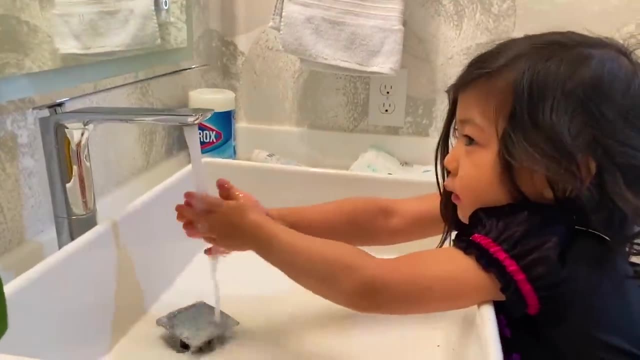 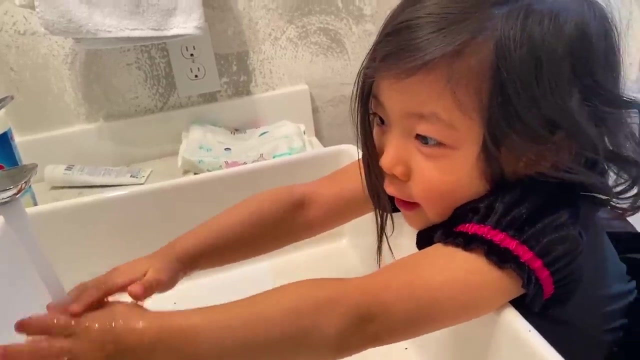 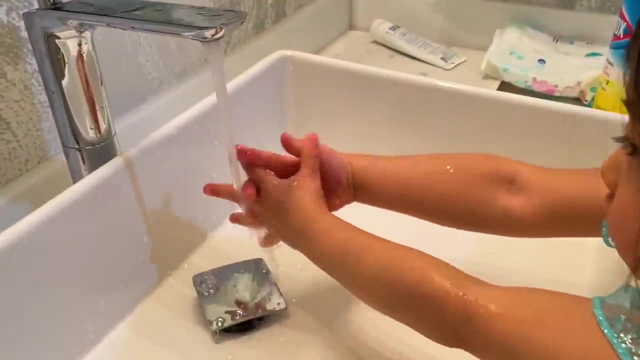 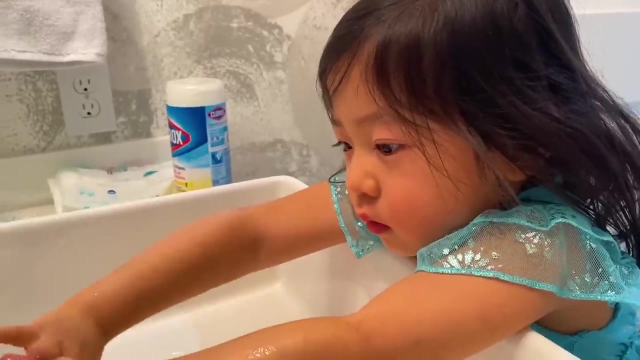 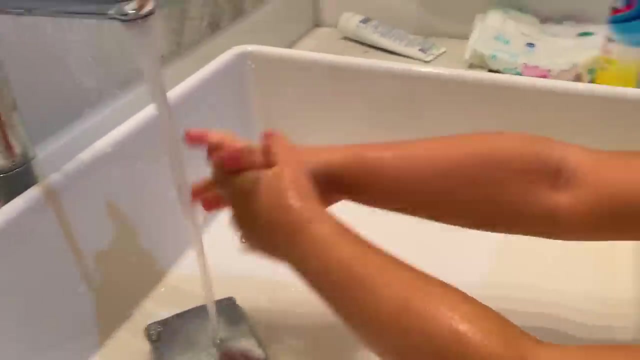 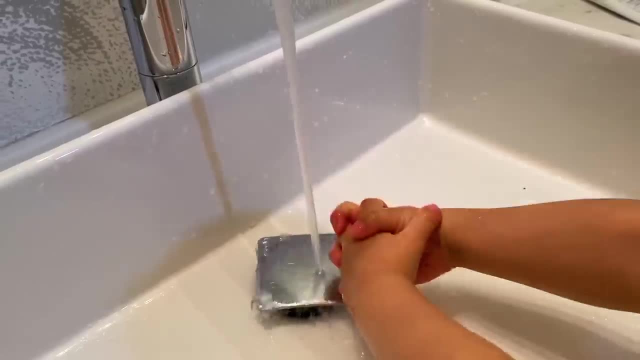 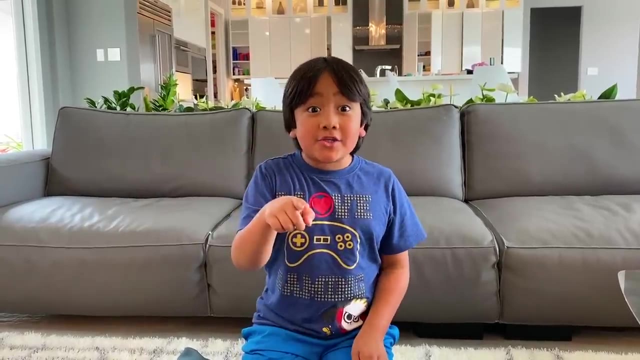 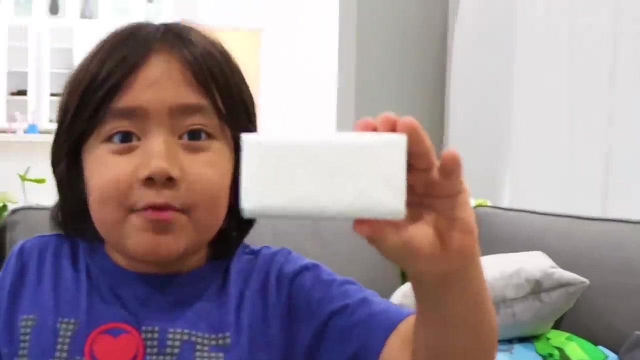 Happy birthday to Emma. Happy birthday to Emma. And that's how important it is to wash your hands. and you should wash your hands, too, for at least 20 seconds. Hi guys, today I'm going to microwave a bar of ivory soap and see what happens. What do you think will? 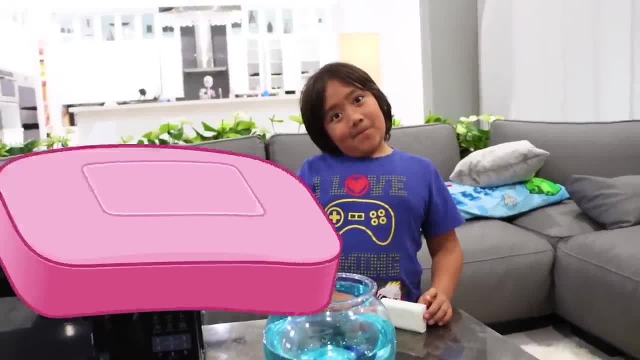 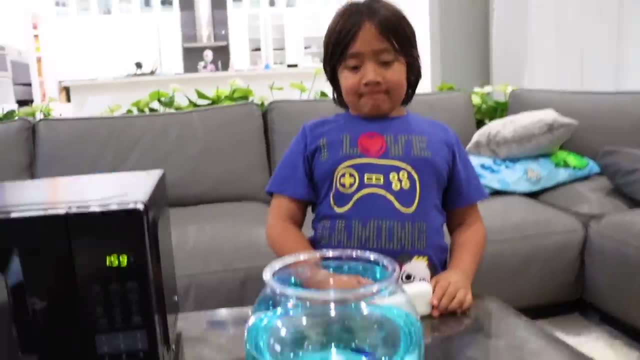 happen, Ryan? Do you think it's gonna melt? Do you think it's gonna become bigger or smaller? Disappear, What do you think? Disappear, Disappear. I guess we'll find out. So what I want you to do first 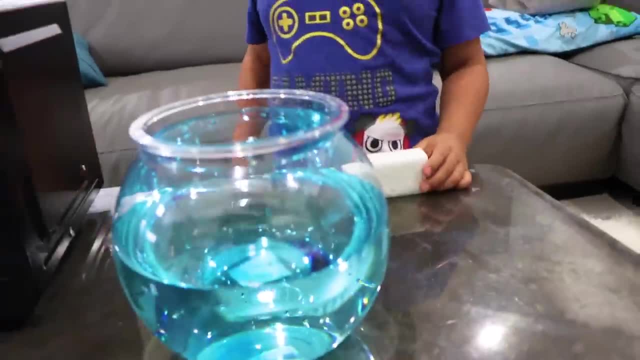 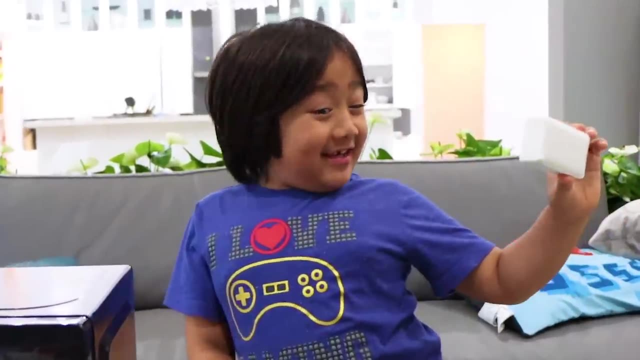 is. I have water here and I want you to put the ivory soap into water and first we're going to see if it's going to sink or not. float okay. okay, do you think it's going to sink or float? maybe float. okay, let's try it. 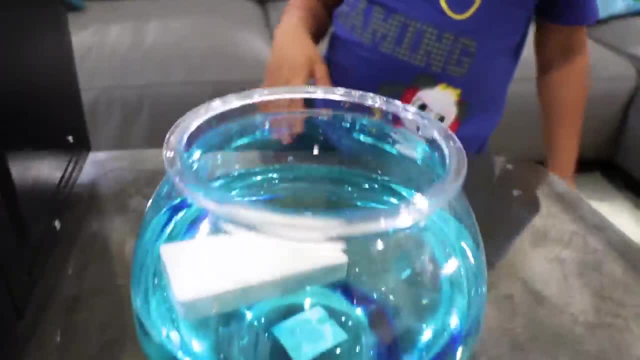 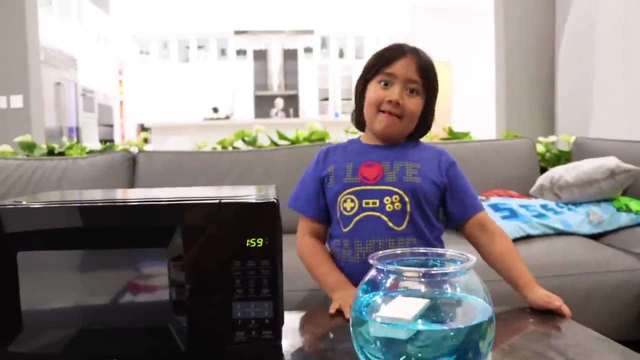 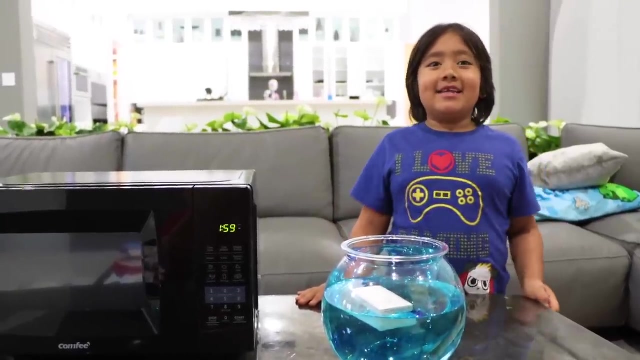 it's floating. yes, there it is. it actually floats in water. we don't have other bars of soap, but if you have a different brand, you can see if it also sinks or float. these are ivory brand. so what does it mean when it floats on water? more dense or less dense than water? uh, less dense, good job, the bar of. 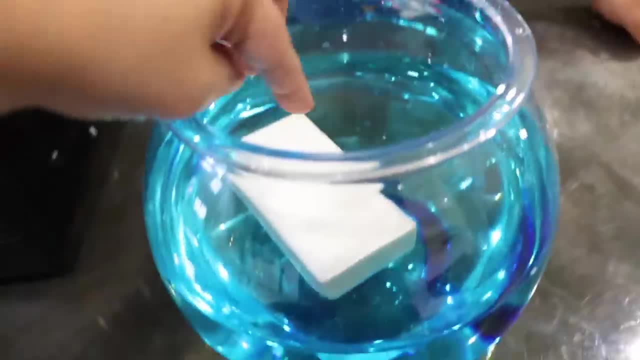 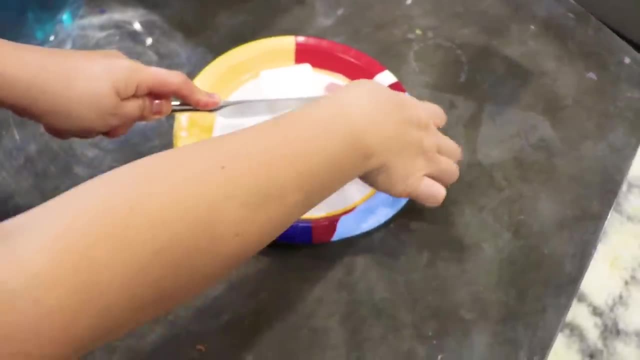 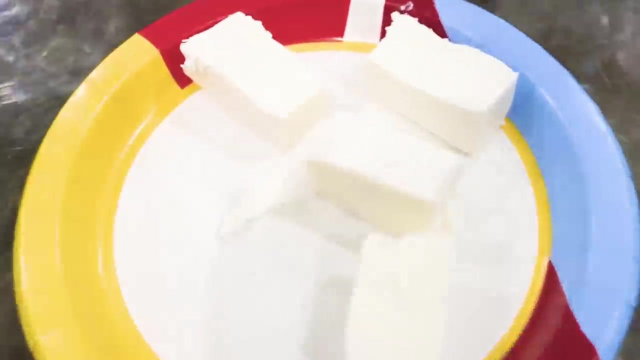 ivory soap, floated because it's less dense than water, probably because there's lots of air holes inside. okay, so we're actually gonna cut it open and see: okay, i'm gonna cut the bar of soap in half. okay, all right, so i cut it more. if you examine it very closely, it has like little holes of. 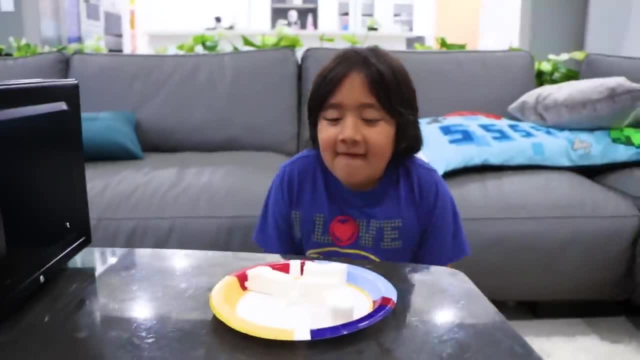 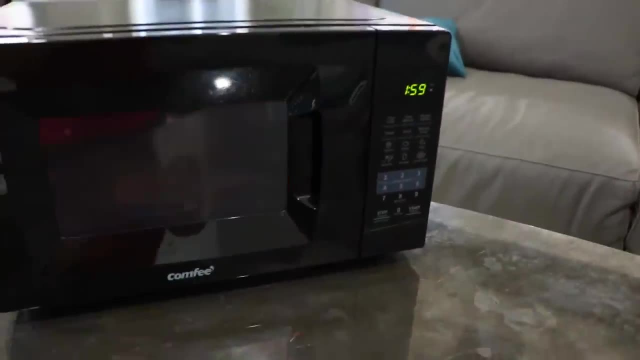 emptiness. i guess it's where all the air is. are you ready to microwave it? yeah, all right. we got our new ivory bar of soap here, put it in the microwave, closing it and it's ready to start. here we go. all right, we're keeping our eyes on the bar of soap. make sure you use a. 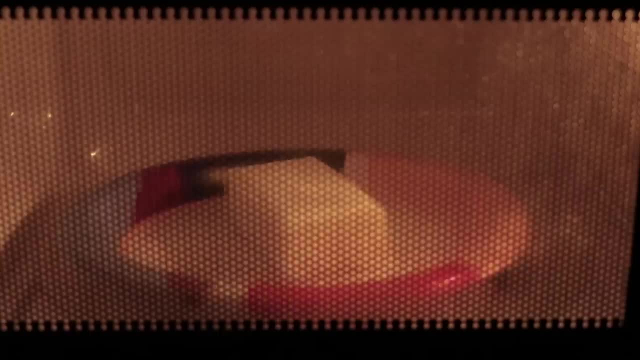 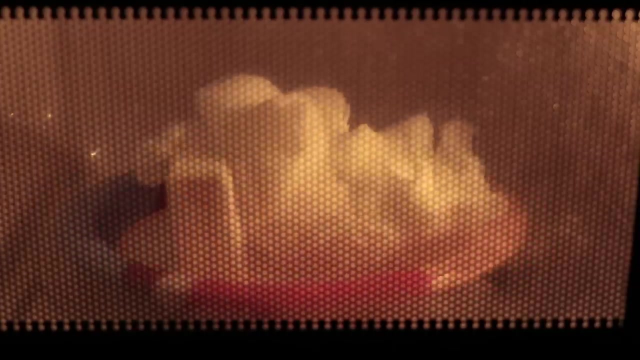 microwavable safe plate. okay, let's see, there's like stuff coming out of it. it's hard to see because you see like the stuff. oh, i do see. you guys see whoa, keep your eyes on it. look guys, it's a little bit hard to see, but look, it's expanding. yeah, it's really by a lot, whoa. 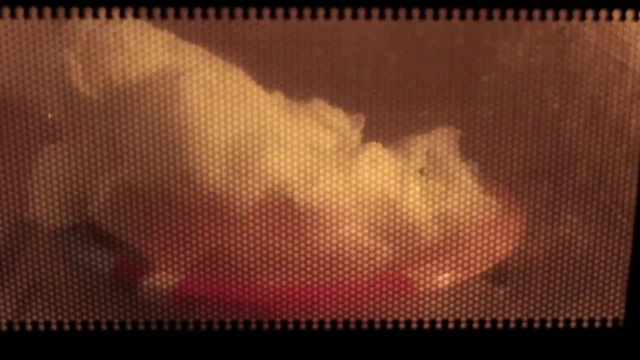 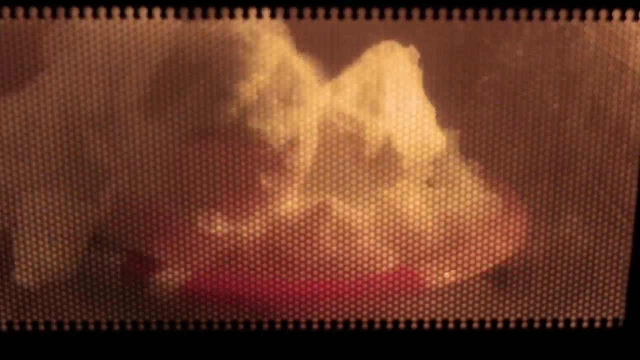 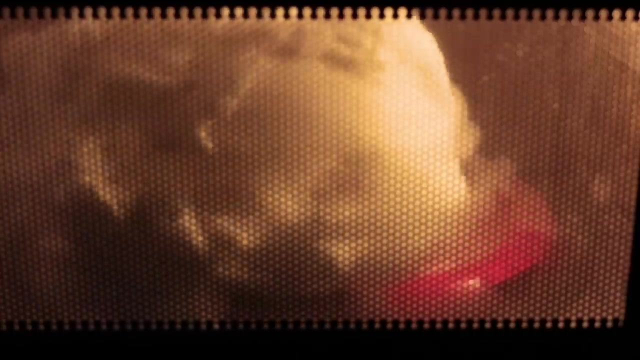 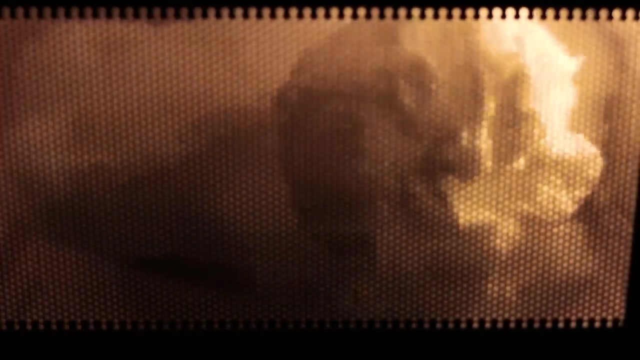 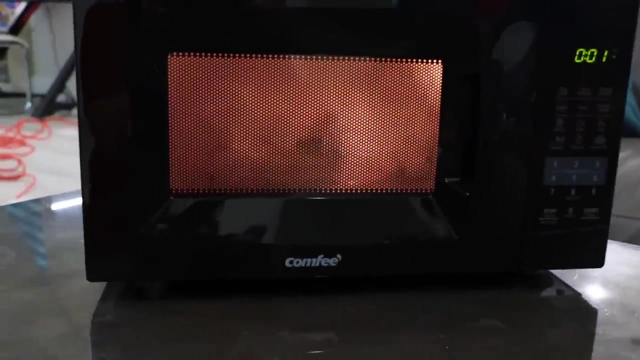 i think it's melting the soap or something. whoa guys, look that's big. should we stop it? it's gonna go all over the microwave. whoa guys, look at this. whoa, whoa, it's like it's the whole microwave. do you smell anything? a little bit smells like soap. yeah, whoa, it looks fluffy like marshmallows. 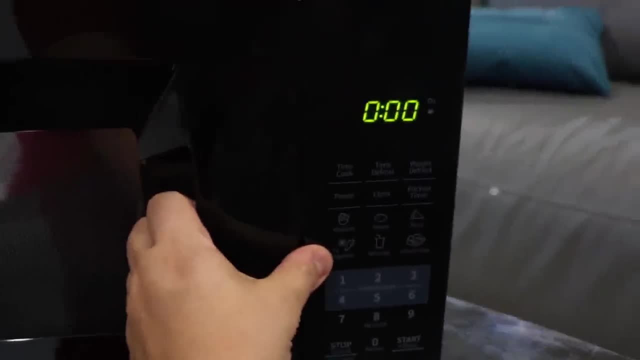 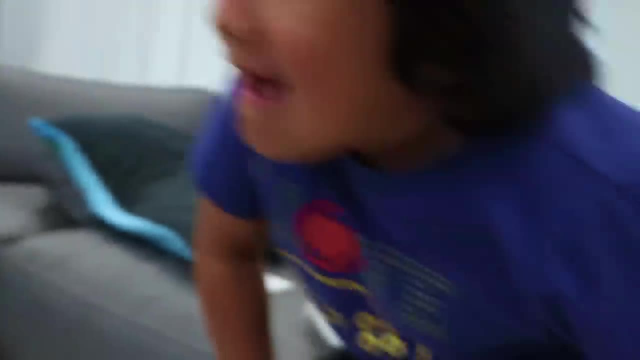 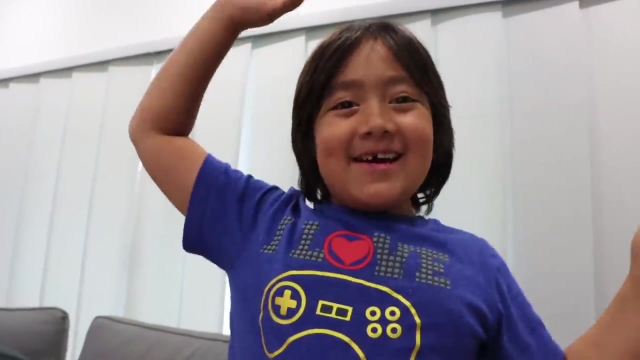 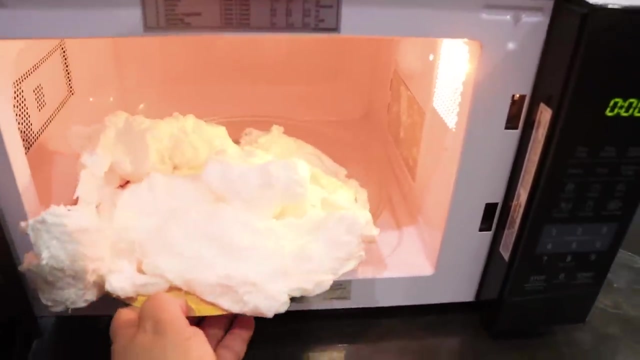 so clean. okay, done, okay, okay. only adults do this, because it might be hot. oh, whoa, did you expect that? no, so what happened? it got melted and then it got bigger. it expanded, yeah, yeah, good, super expanded. look at that. okay, only adult touch this. it might be hot, whoa. 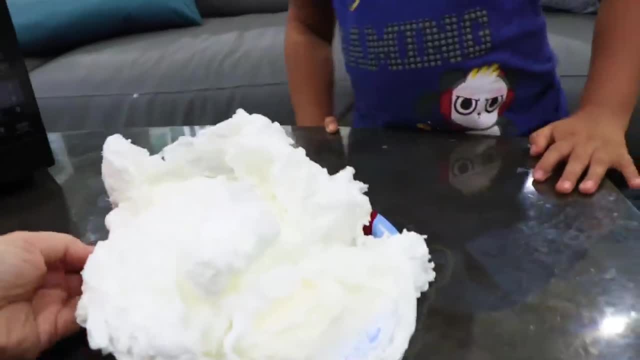 don't touch it yet. okay, it might be hot. okay, we're gonna wait for a little bit. whoa, we're just keeping it 1800 ton to a medium where all that foam is functional. бар be great. this is wow. yeah, Okay, we're going to wait for a little bit. but just looking at it, what does it look? 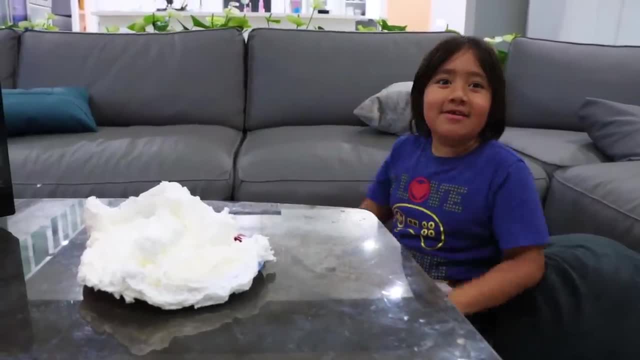 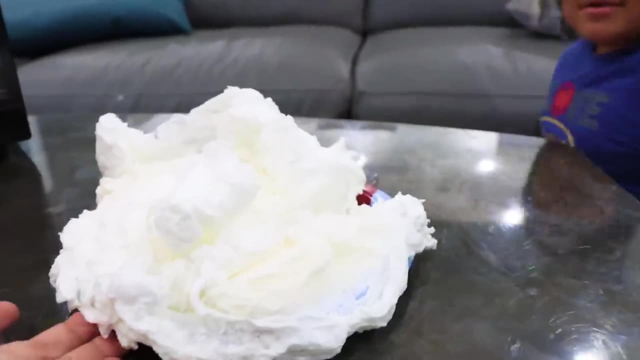 like Toilet paper, Toilets That you like. uh, scramble it a lot, Got it. It looks like toilet paper to Ryan. It looks like a lot, Kind of looks like whipped cream. Yep, Let's see. Okay, so safe to touch now Ryan. 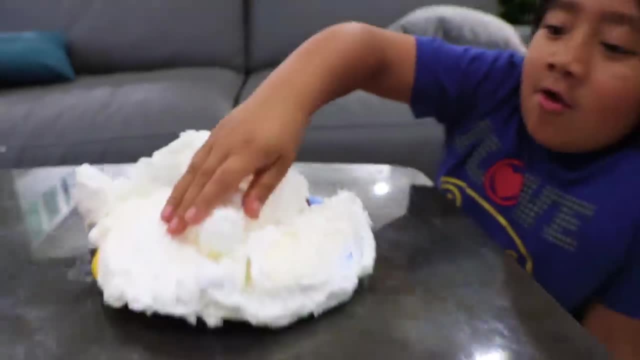 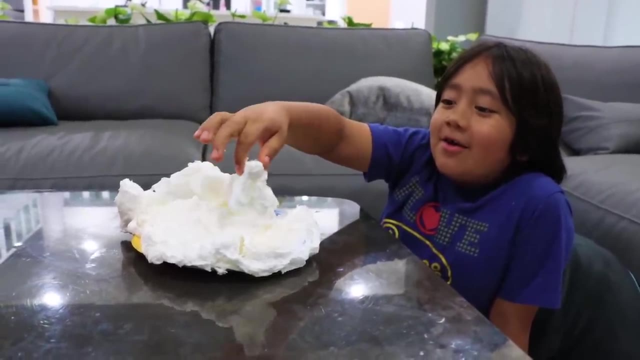 Touch it and see what it Whoa. What does it look like? It feels like maybe, uh, like cotton candy, Really, Yeah, Okay, Wow, It's a little bit more rough, Yeah, so this one actually only works with ivory soap. 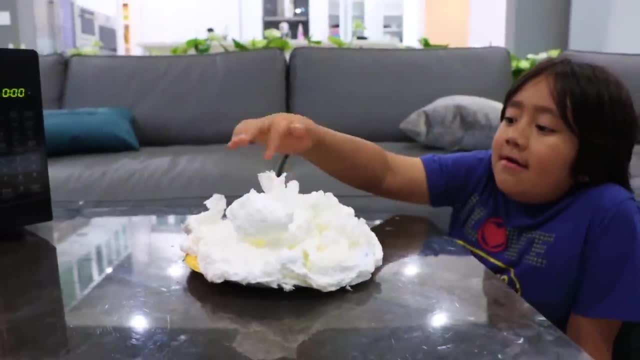 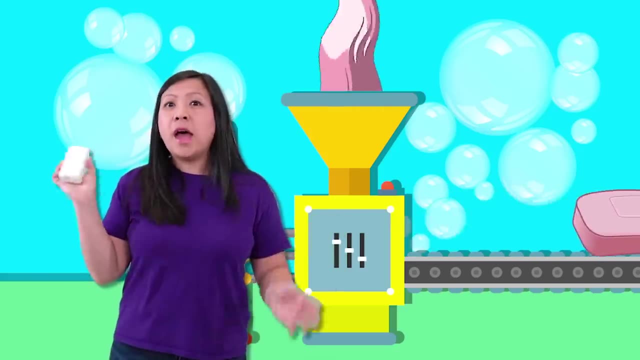 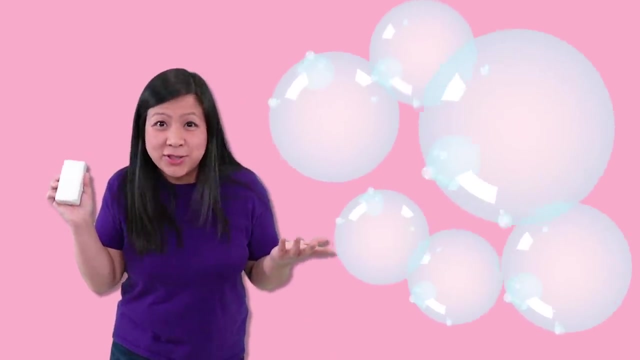 But wait, I don't understand. How does it work? So why did the ivory soap expand in the microwave When it was made? there are air that is trapped inside the mixture And because of the air, that's why it floats in water. 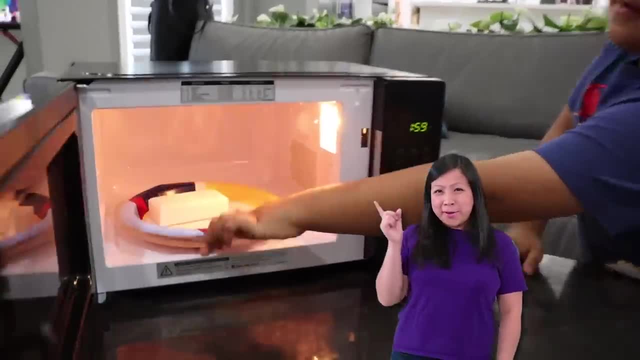 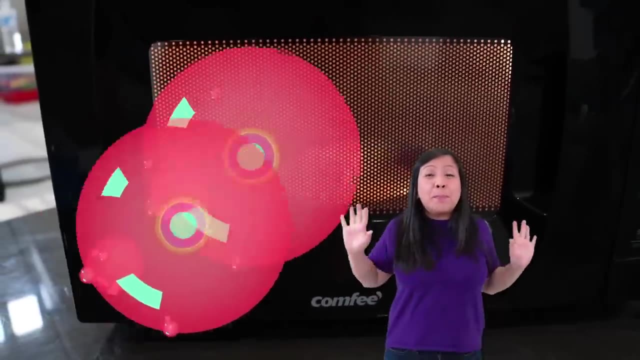 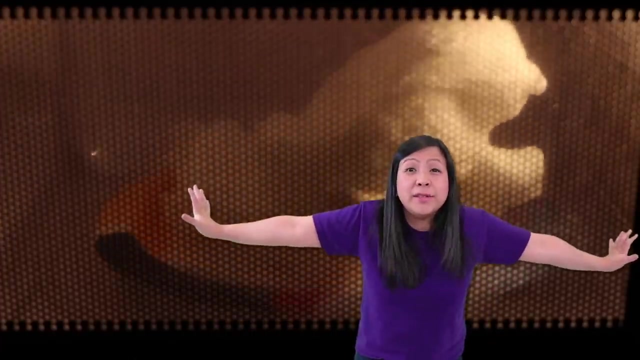 That's right. So when you put the soap in the microwave, the air and the water molecules that was in the soap starts to heat up, vibrate and expand and spread farther apart. They push us against the rest of the soap molecules, expanding the bar into a fluffy. 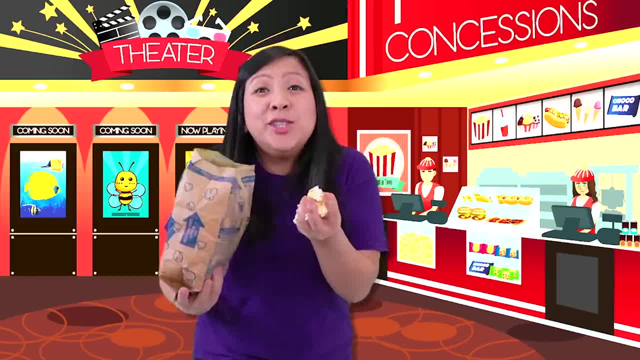 cloud blob. Do you guys like popcorn? It works the same way: Water inside the kernel expands into a fluffy cloud blob. Do you guys like popcorn? It works the same way: Water inside the kernel expands into a fluffy cloud blob. Do you guys like popcorn? 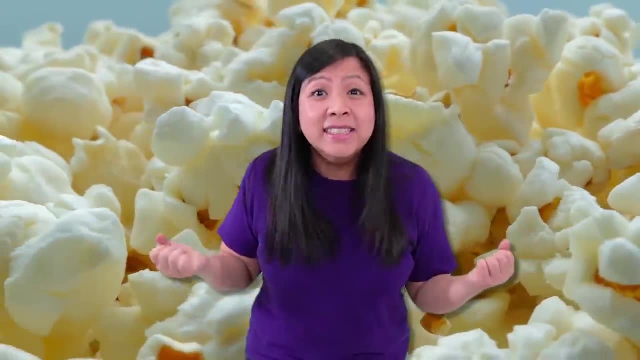 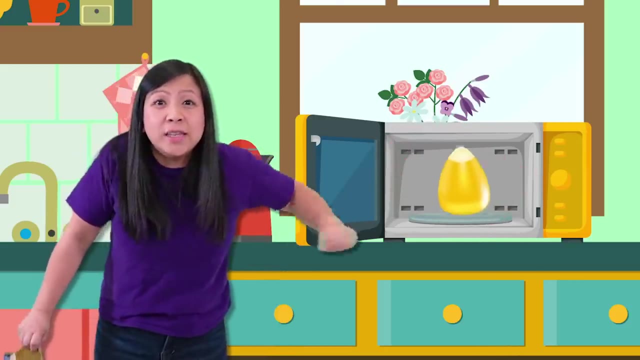 It works the same way. Water inside the kernel expands and pushes on the walls. as it's being heated inside the microwave, The water will turn into steam and expand and pushes along the wall of the kernel until pop, The kernel explodes and we have a yummy piece of popcorn. 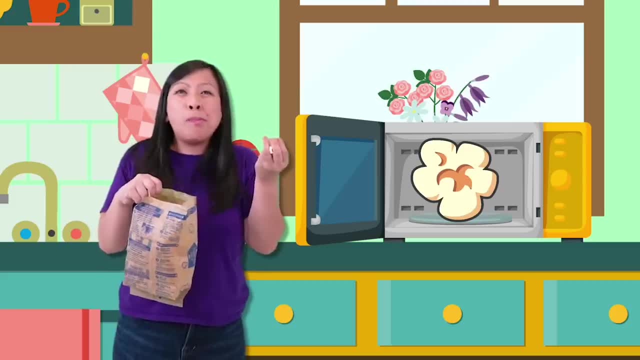 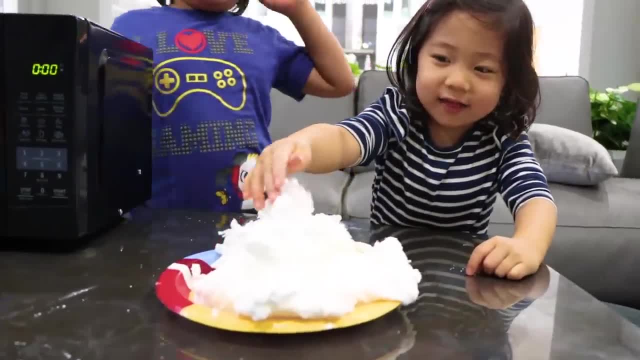 A purple soap. A purple soap, A purple soap. Apparently, It's like coming apart. Why do you microwave it? Well, because I wanted to show Ryan how soap expands when you microwave it. Look See, But it's all mushy. 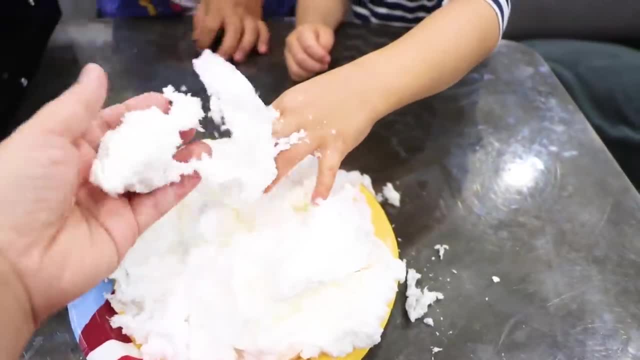 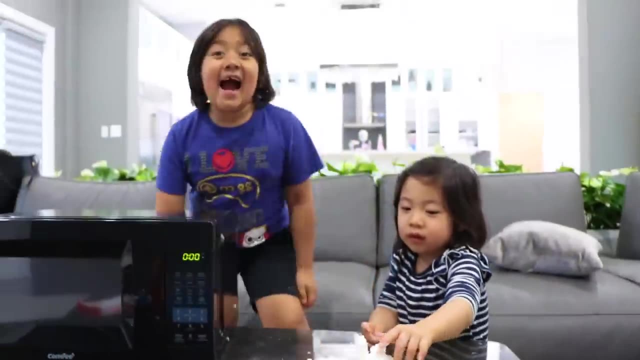 I ruined my fingers. Yeah, but it's okay. It's just soap. We can go wash your hands. Okay, Isn't it cool? Yeah, Bye. Remember always stay happy and rise up. Bye, Boom, Bye, Bye.